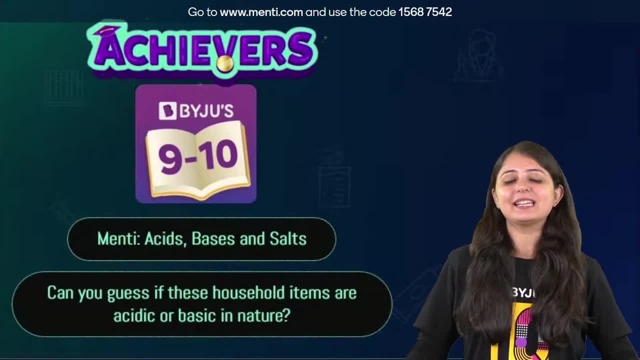 Yes, absolutely. Quickly let your friends know about this. Let's see who knows how much. Who is actually exploring science and chemistry around us? Hey Sanjit, Akshit, Anshita, Tavishi, Dipanshu. Hey, Dipanshu has seen the post on Telegram. Correct, Dipanshu. Hey Raju, thank you so much. Good evening, Gurmila. Come on, quickly give me a green signal that everything is working fine so that we get started. Yes, absolutely. It's going to be a super amazing class. 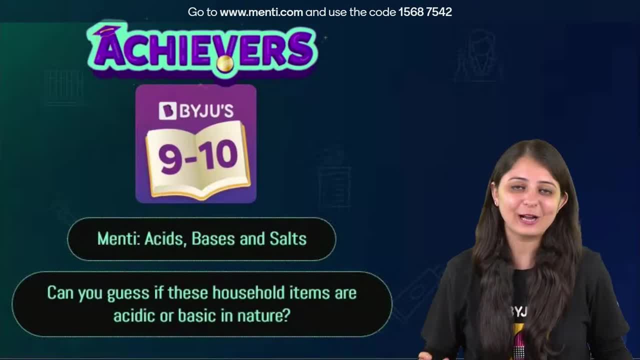 Mendi on household items. I mean, you people keep asking, ma'am, make me a mendi. So there you go. And here we are with another mendi session. Thank you, Sanakshi, for giving me this good to go. 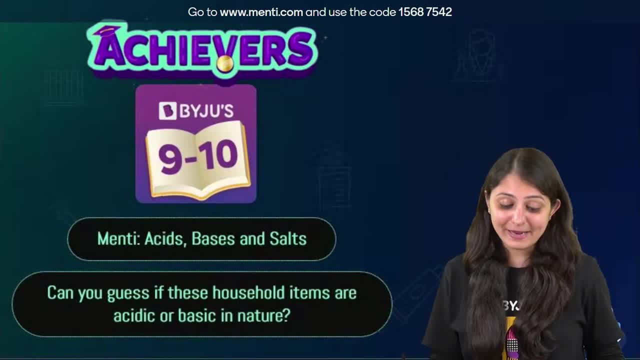 So all of you quickly go to www.menti.com and over there they'll be asking you for a code. The code is 15687542. 15687542. You can see it right there. 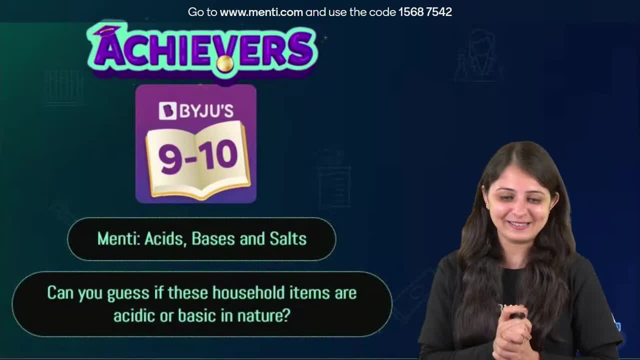 Finally, Mendi. Okay, Innovative26 is saying, finally, ma'am, Mendi is coming. Join. Great, great, awesome. Quickly let your friends also know. Because today's Mendi is a little different. 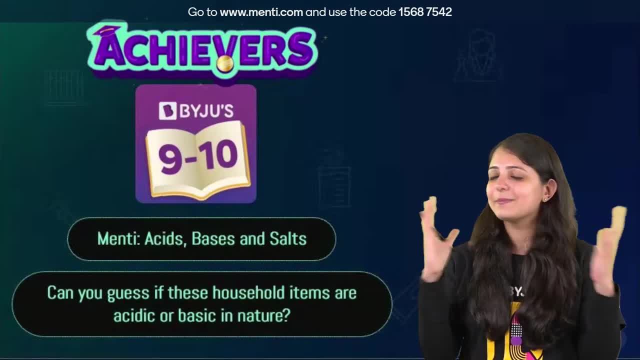 In today's Mendi, you can actually explore a lot of things around you. What you see. What you see. 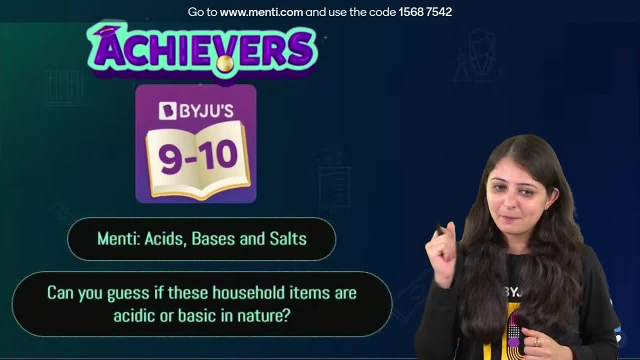 What is acid in it? What is base in it? You will actually understand chemistry in a very good way. No, Gauransh, not at all. The session has just started. From now on, Gauransh is saying, ma'am, you're ignoring it. Not at all. All set for Menti. Awesome. Correct. 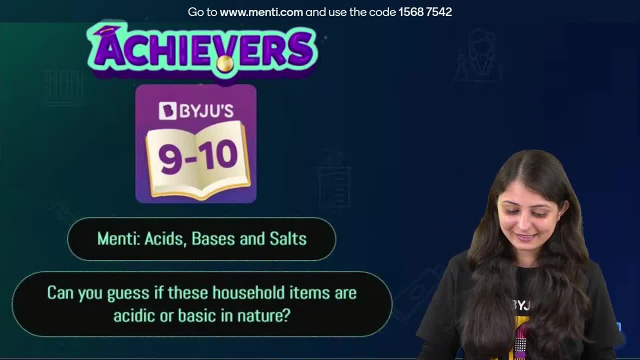 Yes, I can see that. I can see more and more kids are slowly joining in. 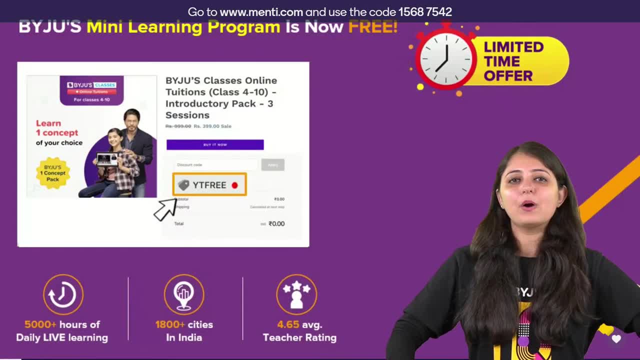 Meanwhile, what we can do is we can definitely tell you about this mini learning program. That's actually. That's actually now for free. So all you have to do is use this magic code YT free. 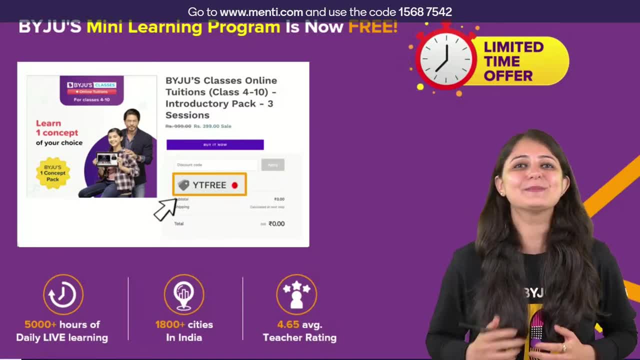 And by doing that, the fee would be waived off. And this is for a limited time period. So quickly, after the session, if you haven't tried this, go ahead and grab this opportunity. 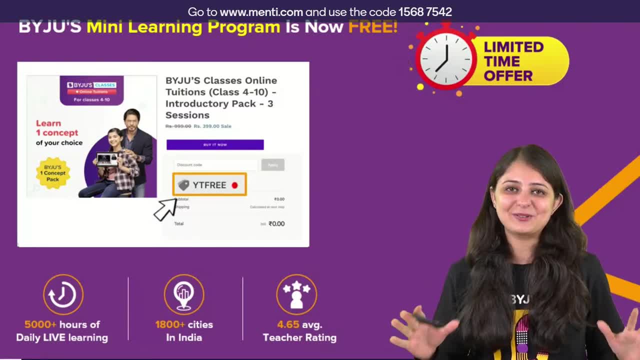 Yes, Anoop, there would be a lead award. I know you people get all excited. Who is leading the lead award? Hey, cute world. Good evening. Always ready for Menti. 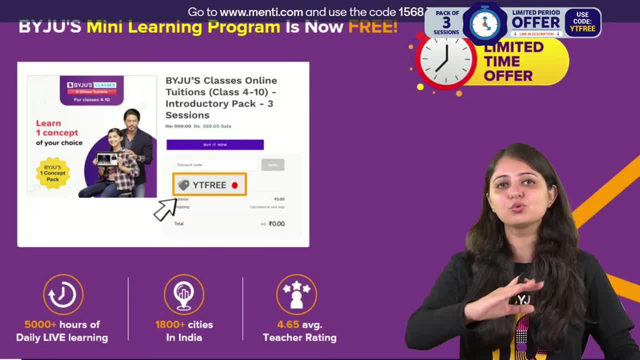 Manasvi. Okay. Hey, Adhiraj. Adhiraj is super excited for Menti. 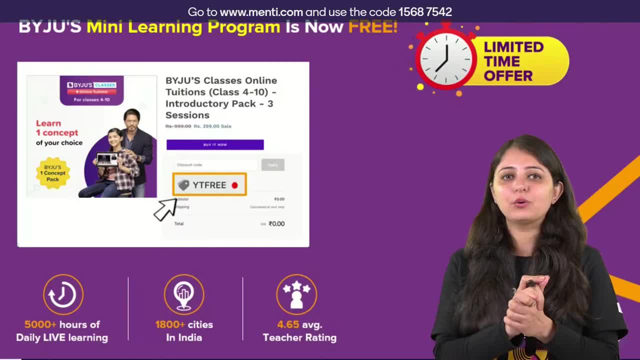 Okay, tell me who has tried the YT free code and how are you finding it? Because your feedback matters to us the most. 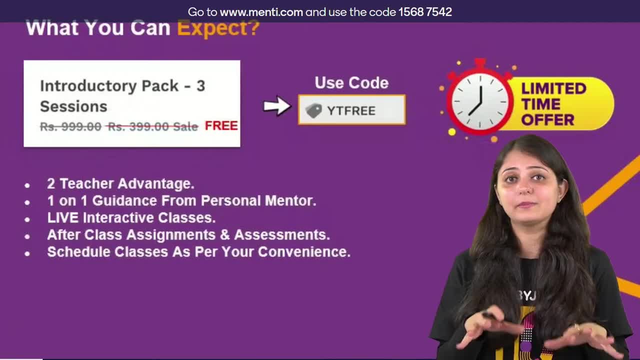 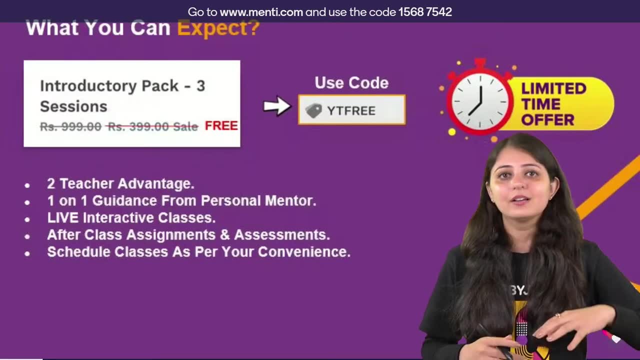 Yes, because if you've actually explored this, you'll realize that you're able to unlock so many premium features. You'll get the introductory pack of three sessions for free. There you can see two teacher advantage, live interactions. Live interactions are happening. Assessment questions are there. 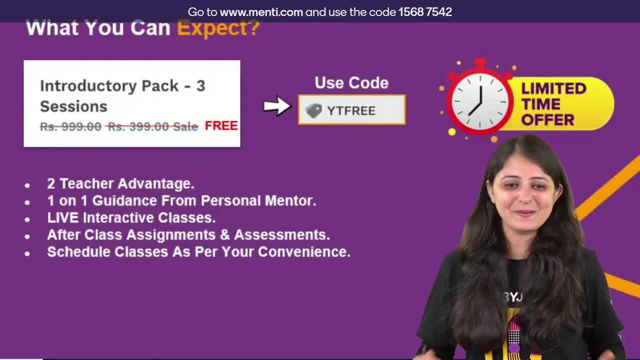 You can schedule the class as per your choice. Choose the topic. Manasvi, technical sir. 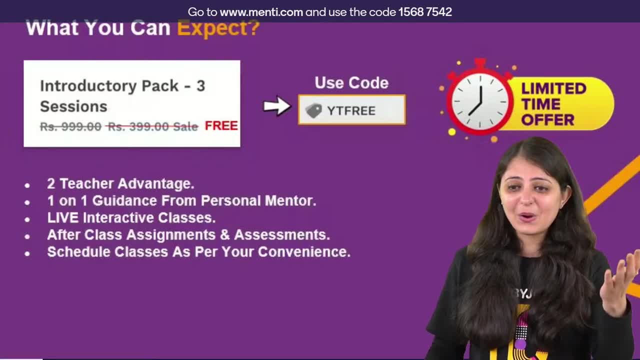 Pagalapati, Rosaina, Vaibhavi. Good. Good to see. So many of you have tried and you've liked it. Very useful. Good. 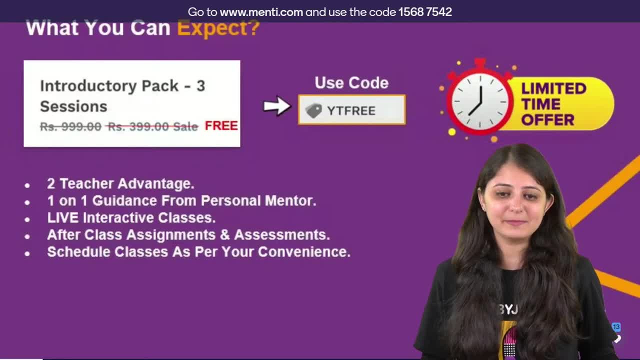 Muskaan is curious. Super curious for this Menti. 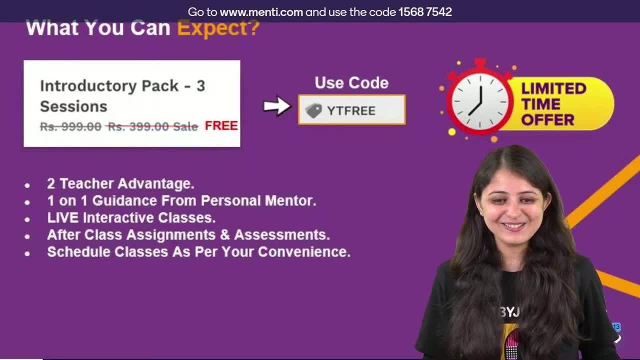 Nice. This is good. Hey, Jatin. Good to know that. All right. 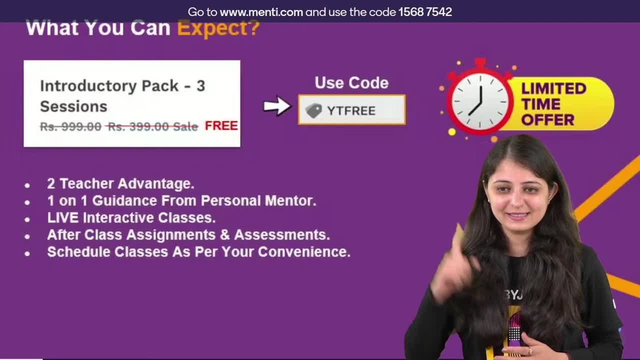 So, I hope all of you've joined the Menti that we are having. Great. 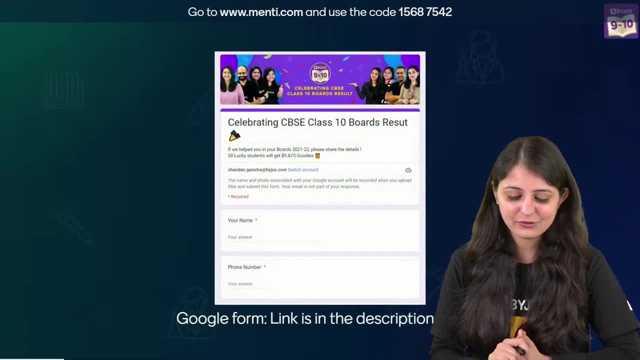 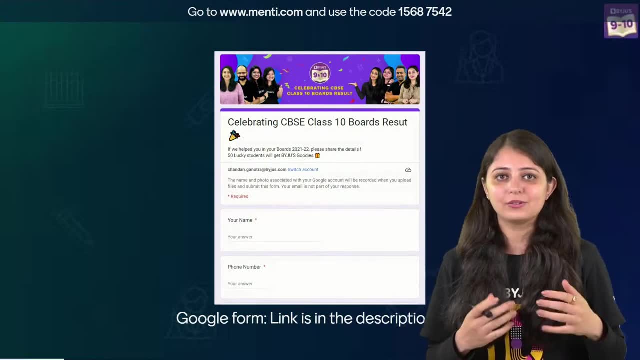 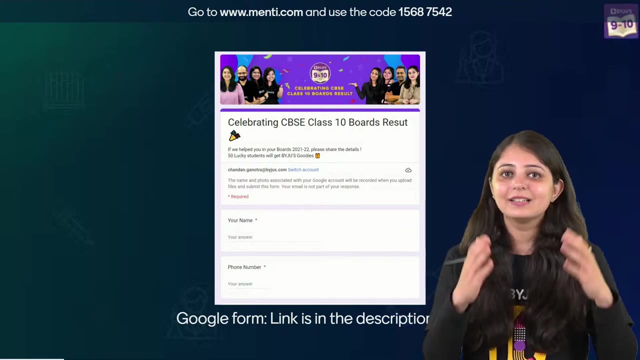 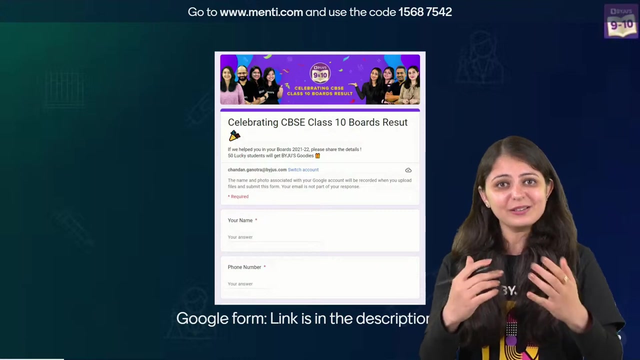 But before we get started, there's something really interesting for all of you. So, if by any chance we have any ex-10 graders with us or you can, you know, let your siblings know, let your neighbors, cousins, everybody know. If they were a part of our journey in 2021-2022, that academic year, if they were with us, we would definitely want to have, be a part of the celebration of their board result as well. So, quickly let them know that there is a Google form in the description box. You can, you know, pass this form to them. 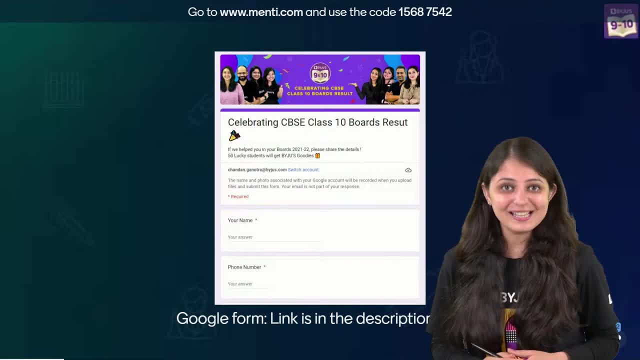 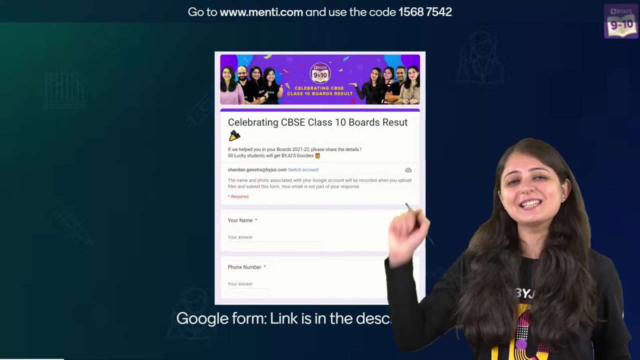 Ask them to fill this form because 50 lucky winners are going to get buy juice goodies. So, yes, maybe your sister, your brother, cousin, neighbor, whosoever was there in the last academic year. That is 2021-2022. Ask them to fill this simple Google form. And yes, then there's a chance that they can win the buy juice goodies. 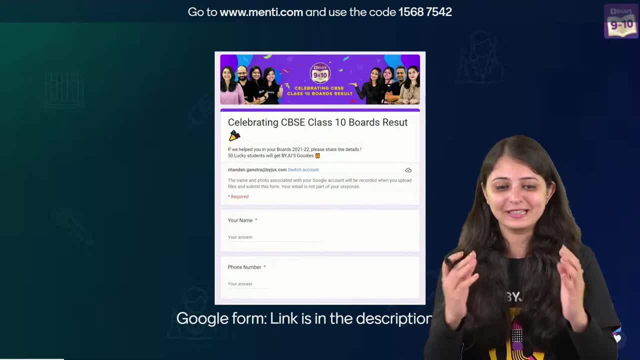 Yes, yes. I'm waiting for a minute. Cute. Will you quickly join in? Absolutely. Absolutely. Okay, we will definitely wait. 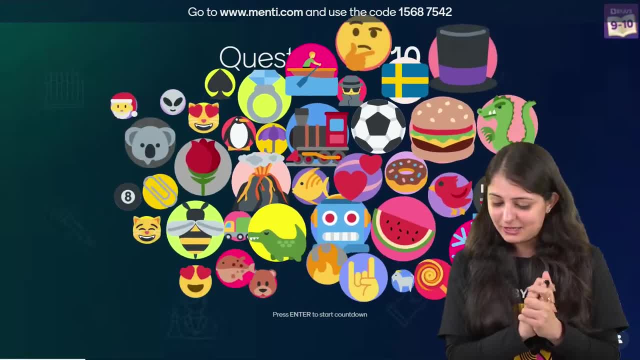 Till then, let's just tell you the rules. Okay, let me just explain you the rules. 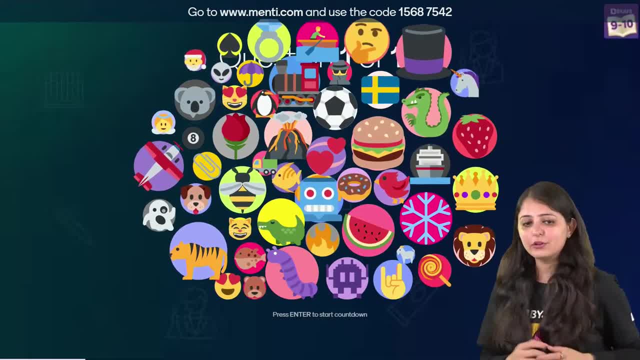 So, we'll have 10 questions in all. I'm waiting. Don't worry. I'm waiting for you to join in. We'll have 10 questions in all. 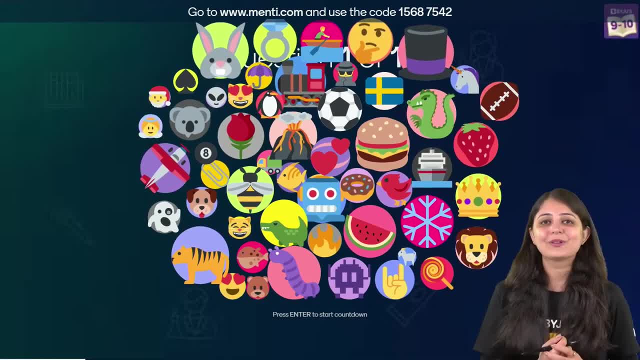 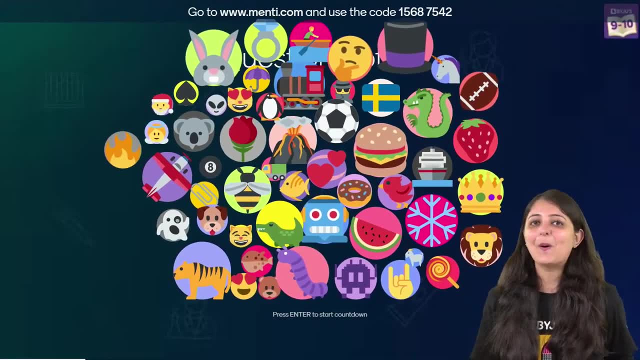 Okay. And we have 10 household items over there. For every household item, you have to just make a very small decision whether that household item is acidic or whether it is basic. 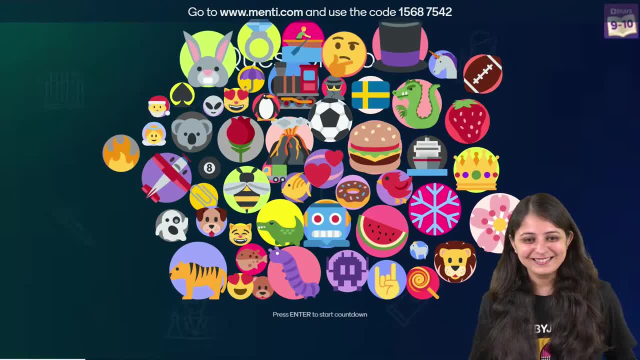 Sounds like a really basic question, right? 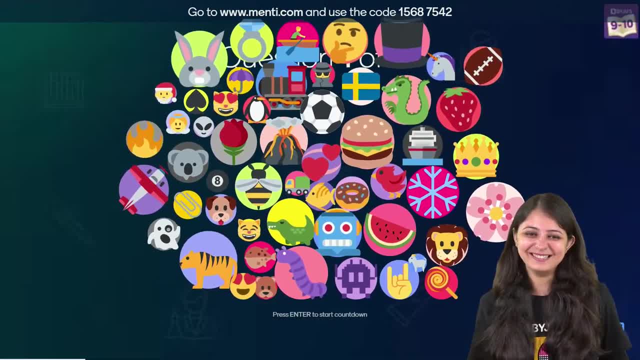 Hey, Muskaan, if you're appearing for the votes in this academic year, then not. 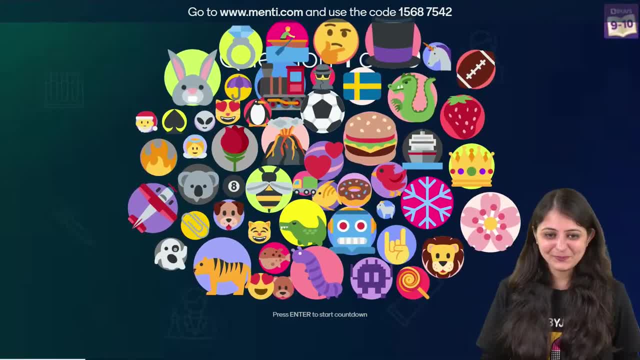 Okay, you're a burglar. Hey, Prisha. So, your options are very simple. 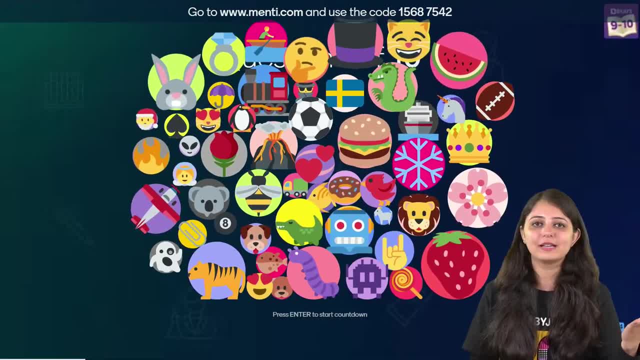 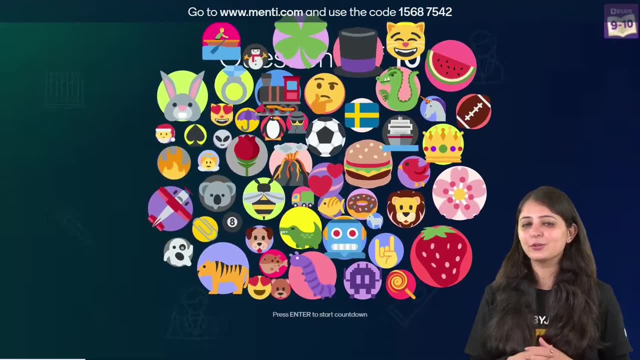 Very sorted mentally this time, right? You'll have one option as the acidic nature, one option as the basic nature. Okay. So, it's going to be very sorted when it comes to the two options that you have. 50-50 chance and this time, I'm really hopeful that most of you will get the answers right. Can I have that kind of trust? Tell me. Yeah, I can see that. Nibha, okay. 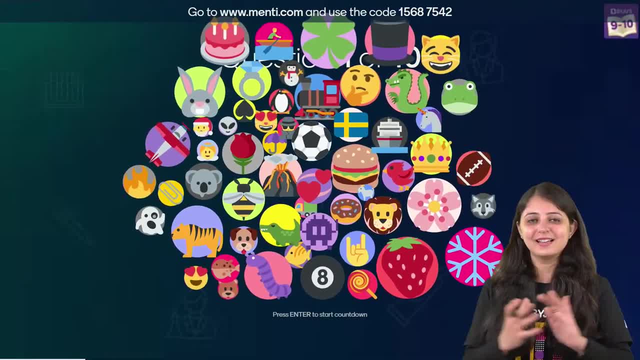 Okay, Nibha noted. Nibha, I hope you're there on the leaderboard. Yes, you are. Great. 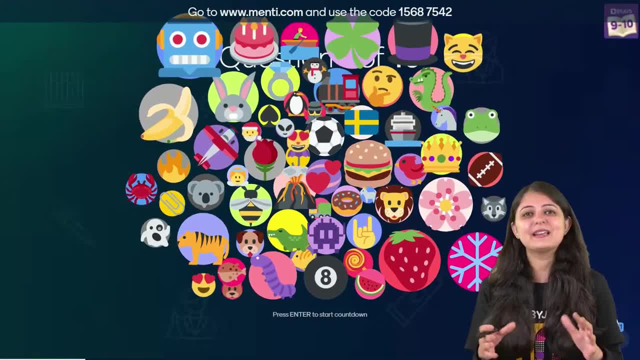 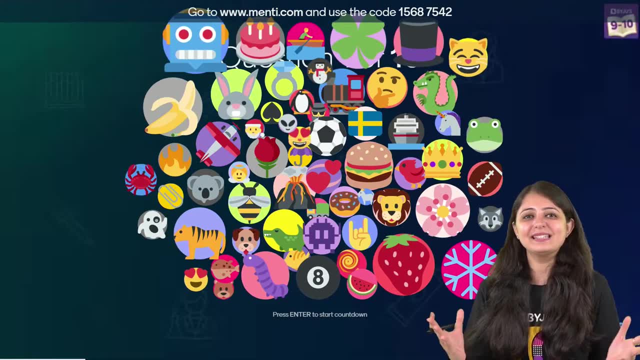 So, I keep telling you, explore the magic of chemistry, explore this. Now, I'll check. Are you actually, you know, trying to explore the science, the wonderful world of science that's around you? Yes. Yes, Anju. Absolutely. Really important part, right? Yes. Yes, Nibha. That's the spirit. 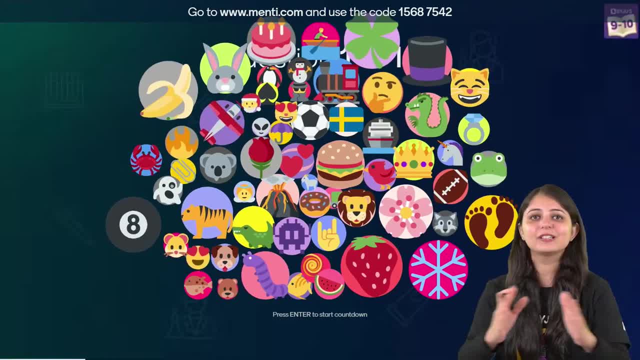 So, Nibha is saying, I'll make sure that I'm there on the leaderboard. Awesome. Bunny. Okay. 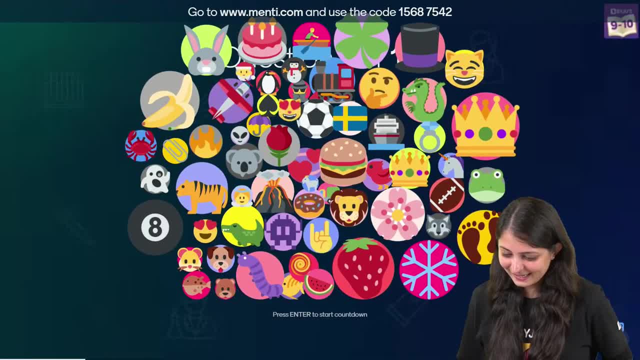 Yes, definitely I can see, I can see that. All right. All set? 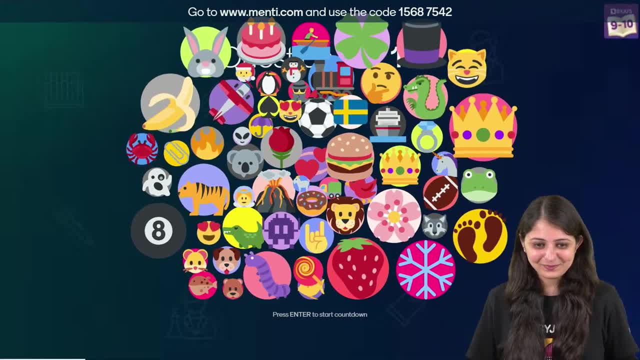 Eagerly waiting for the first question? Excited? 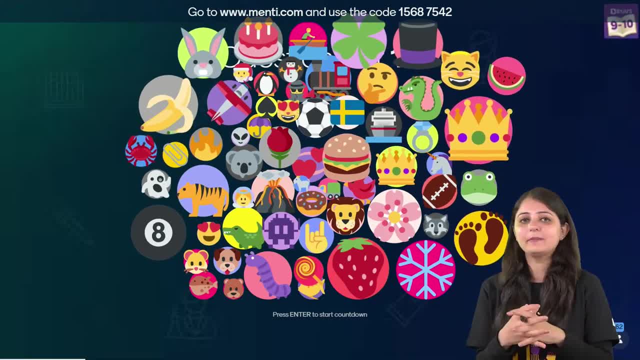 So, you know, for this particular menti, I know you'll land on the correct answer. Where is we? We explore the items that are around us. 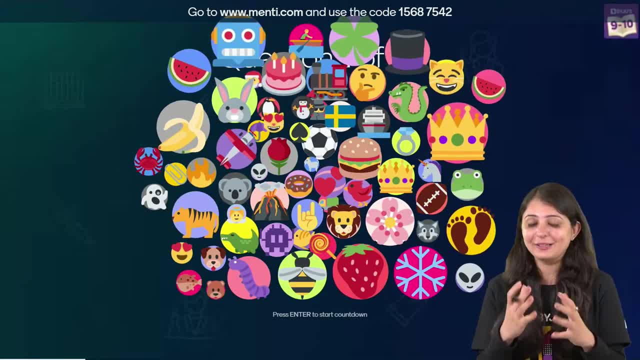 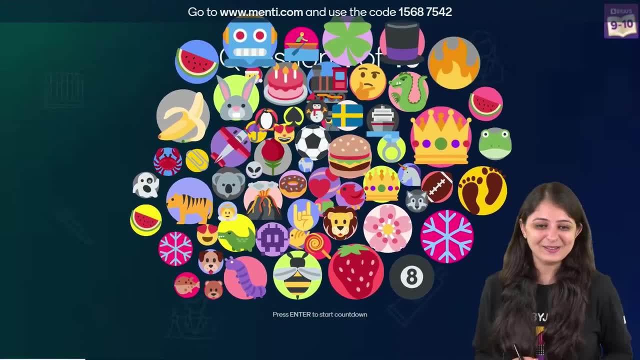 Now, the question is, who's going to do it quickly? Correctly, I'm taking it for granted that you might do it. Who will do it quickly is actually going to tell us who's going to come on the leaderboard. Yes, Webavi. Let's get started. All right. 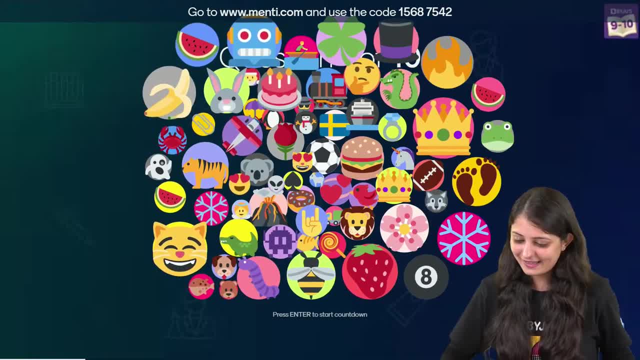 So, we have a lot of kids with us now and then it's perfect time to start now. Yes. All right. So, there's one small question. Yes. All right. 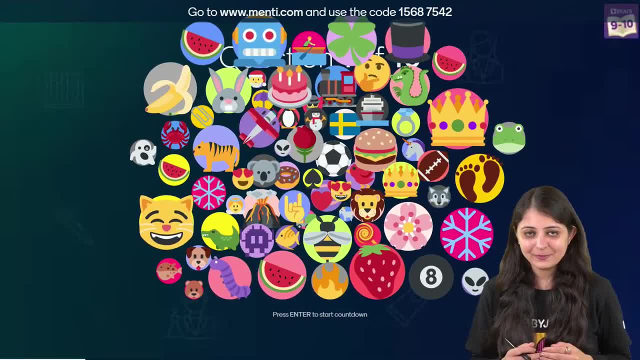 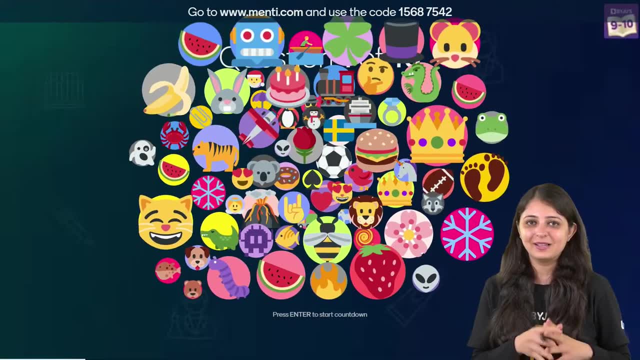 So, there's one small rule over here. After every question, I want you to tell me what exactly was your rank. 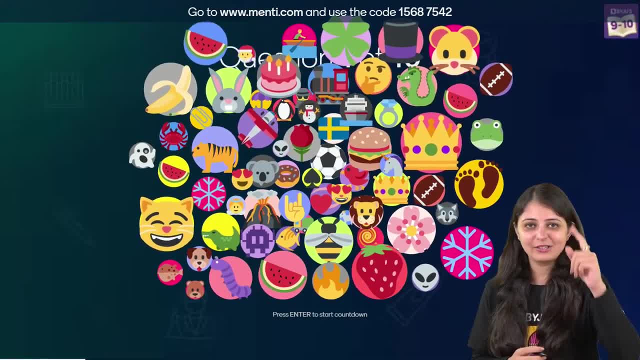 If you get the rank after every question or is it after the leaderboard? After the leaderboard. Okay. Okay. 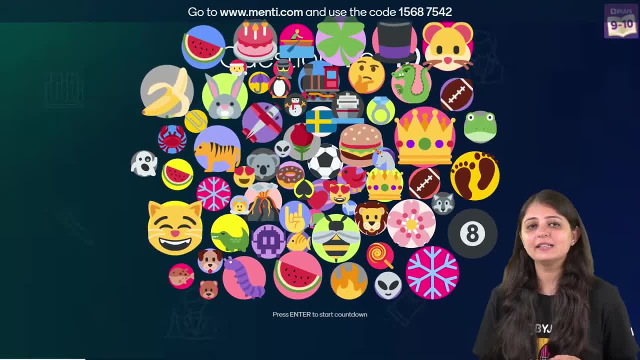 All right. So, simple rule. After every question, if you get that question right, I want you to give me loads and loads of thumbs up. Simple. 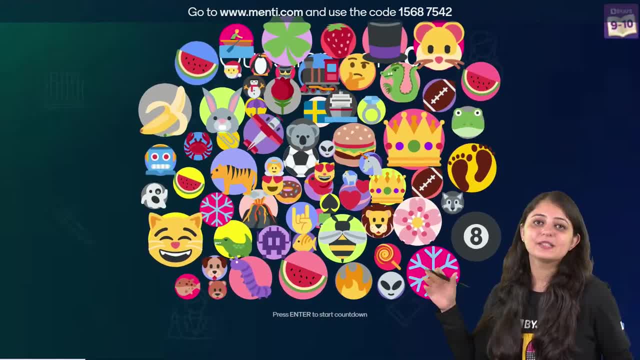 This way, I'll get to know that okay, maybe you didn't give the fastest answer but at least you got it right. Adirajah Singh. Okay. Okay. All right. All right. We've got a perfect 70 on the screen. Let's get started now. Okay. 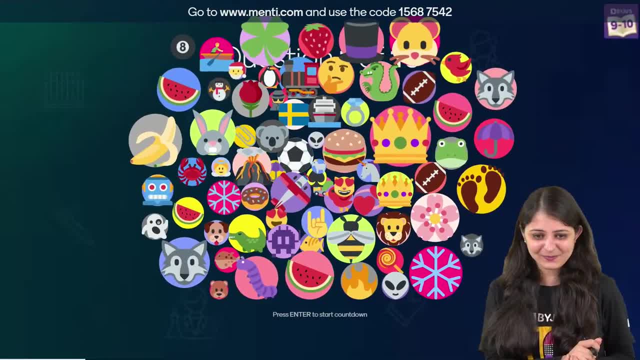 Webavi Singh, no answers in Tacharya. That's also like a good rule that we can have. Once you're done with the question, you post done, you post the, you know, the time, timeframe in which you've answered, maybe one second. 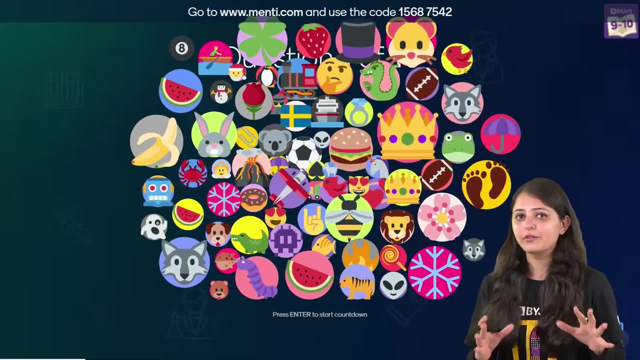 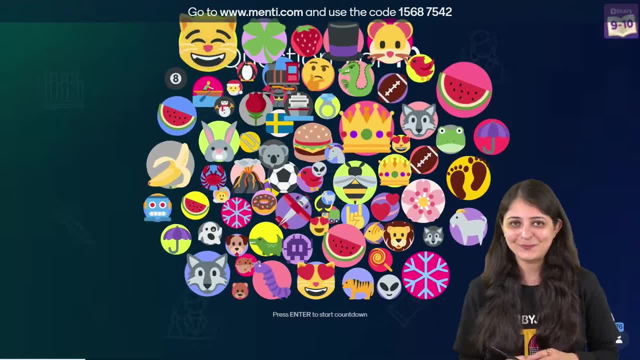 Maybe one second, two second, five seconds but let's not post the answers here. 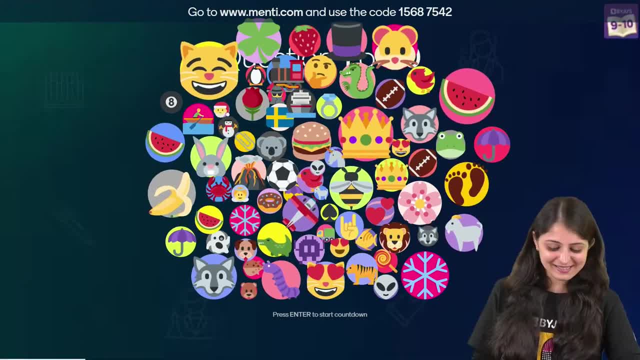 Okay. Correct? Start. All right. So let's get started. 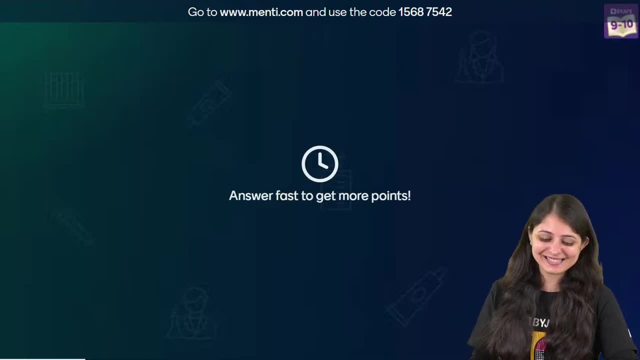 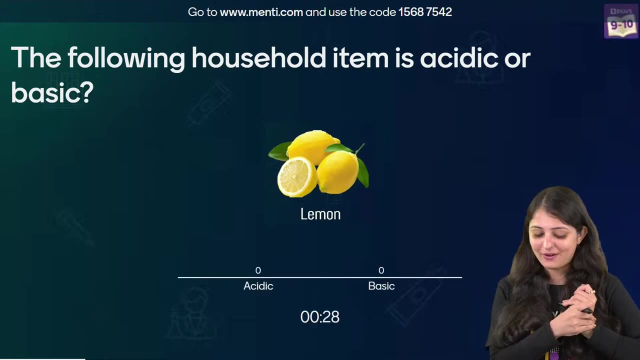 The first question is on your screens Now. The Follwing household item is acidic or basic in nature. That's what you have to figure out. And they have given you the first household item. lemon. Ruzaina already gave thumbs up. That means she's attended the questions. 0.9 seconds. Done. 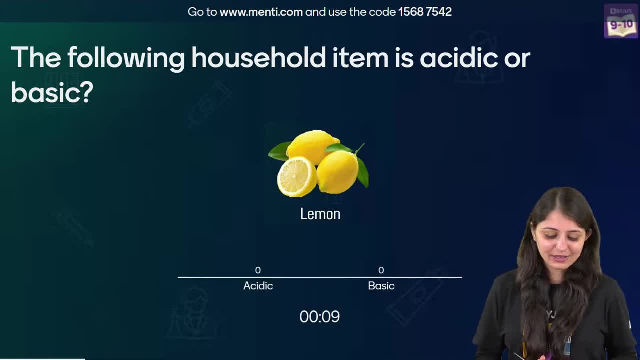 Super easy. Great. You're still left with 10 seconds. Get this one right. Lemons. Are they acidic or are they basic? 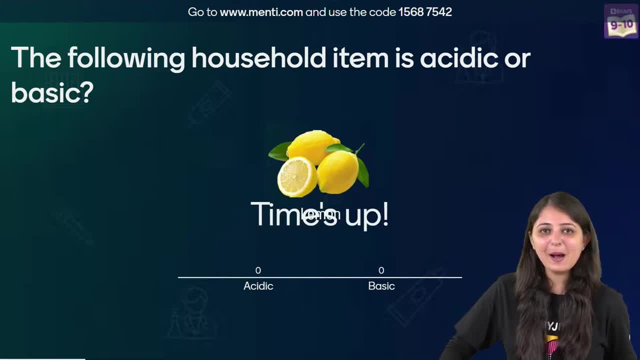 Yes. Let's see. Time's up. Let's see how many of you got this one. 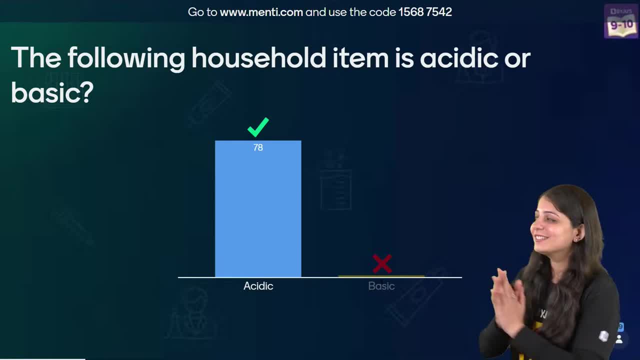 78 of you got this one right. Well done. 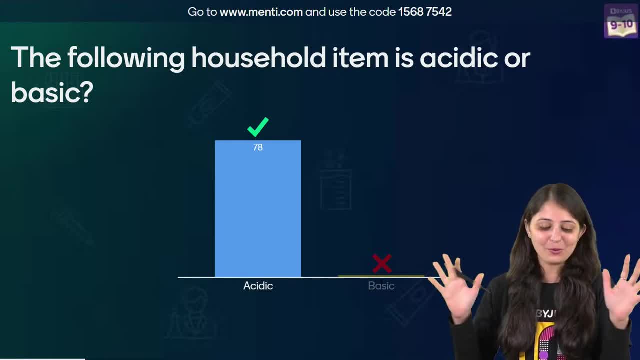 This is like a super happy scoreboard right now. Good. Awesome. 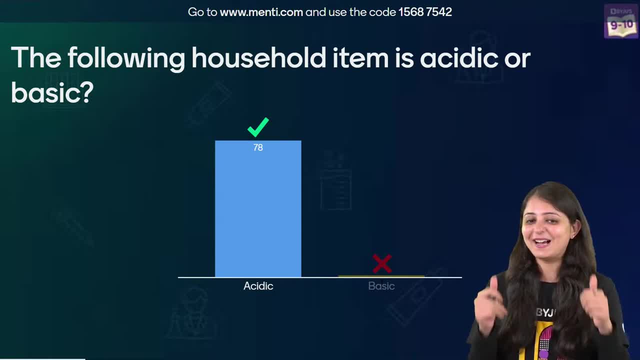 I mean I'm going to get 78 thumbs up here. Muskaan is the first one to post that thumbs up. Good. 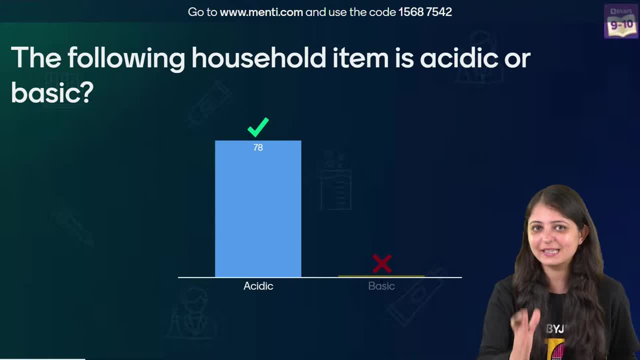 Great. Yes. So the moment you get the question right, I want to see that kind of excitement in the chat box as well. 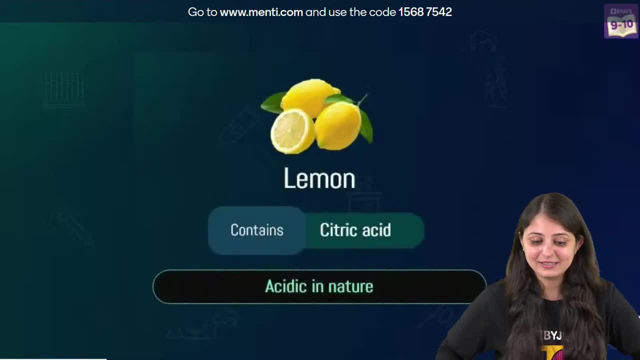 Alright. Yes. You people have guessed this right. Lemon actually contains citric acid. 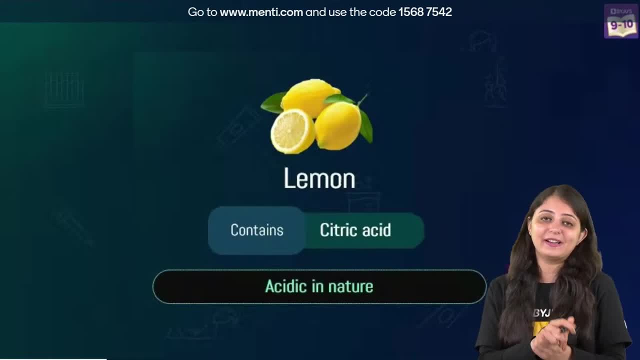 In fact, all citrus fruits, they contain citric acid. So you'll find it oranges also. You'll find it in berries also. 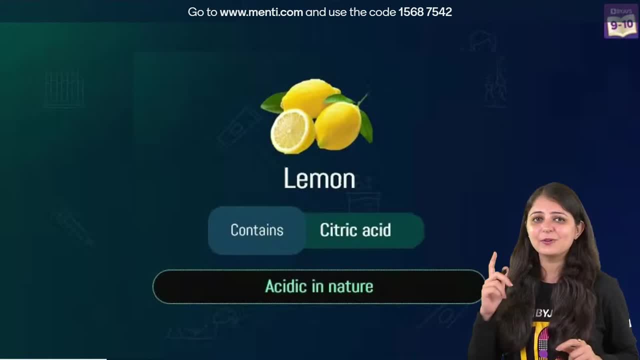 By the way, we discussed this yesterday. What is citric acid? Organic acid or mineral acid? Come on. Tell me in the chat box. Is it organic? Is it mineral? 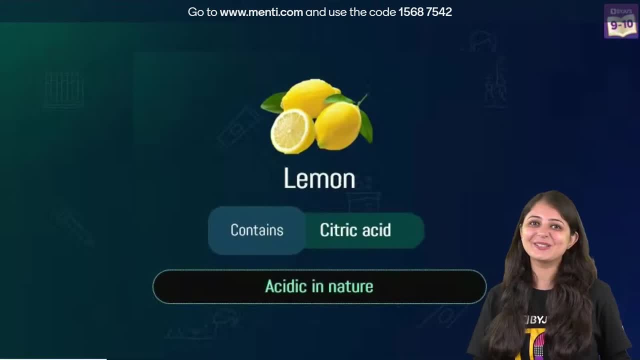 Today, it's going to be a very good competition because I'm really curious to see the leaderboard. 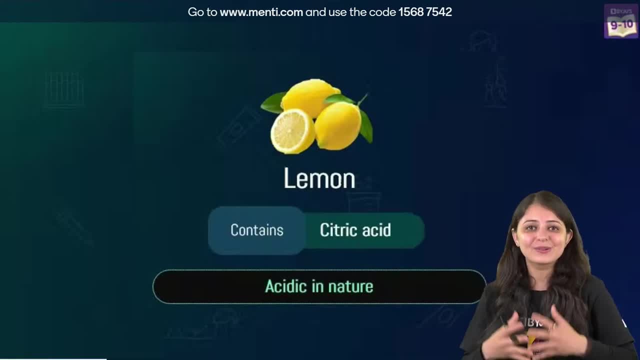 Organic. Correct. Correct. So, plants and animals get it from natural sources. Weak organic acid. Correct. Absolutely. Right. All of you 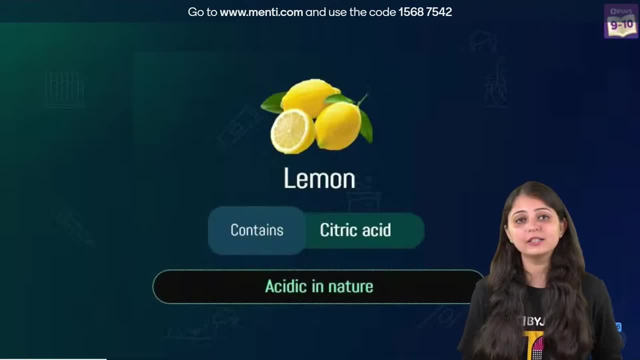 are super confident at this point of time. It's so good to see the chat box. It seems as if only one person is commenting. Because all the comments are the same. No, I'm not ignoring anyone. Not at all. Alright. 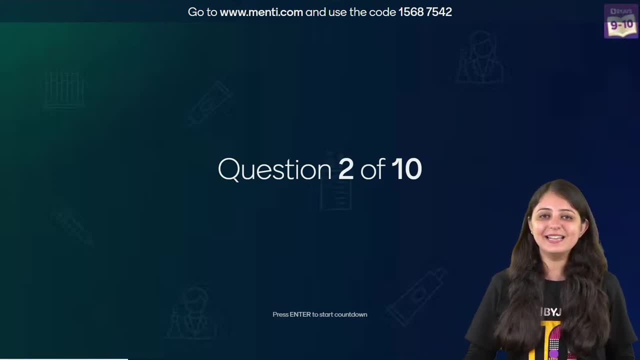 On this positive note, let's load question number two. 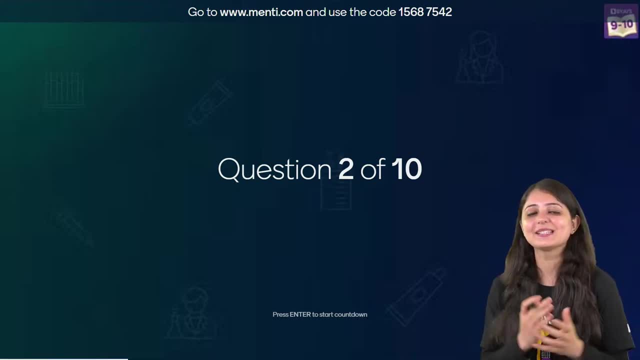 Again, be really quick because you might have come across this household item. 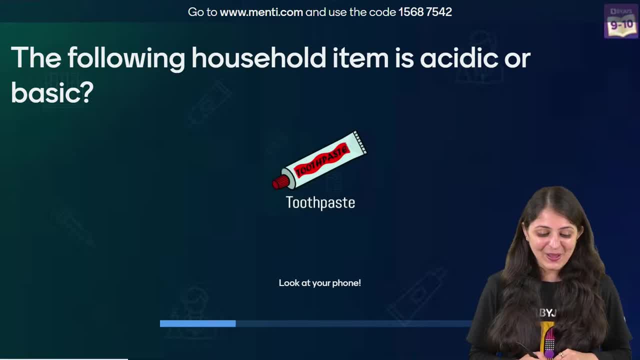 and accuracy. That's your focus. So, the second household item that we have for you is a toothpaste. Well, we use a toothpaste, right? But do we know why we use a toothpaste? 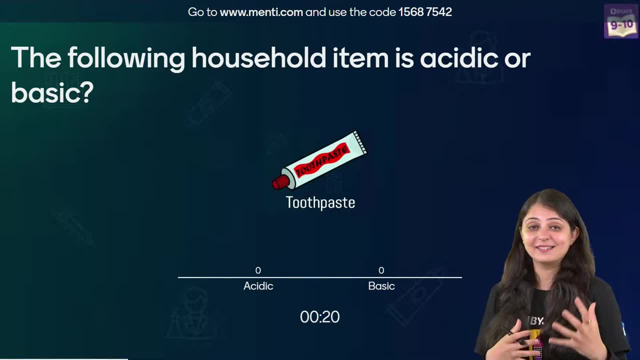 Just parents said to brush it or there is a reason. There is a science behind this. There is a chemistry behind this. Everyone has voted. So, even the 30 seconds we are giving, Menti is also saying, why 30 seconds? Zero. They are super amazing kids. Just make it 10 seconds only. 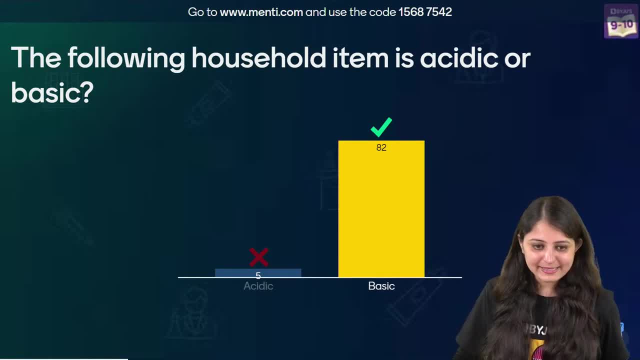 82 of you got this one right. 5 kids also voted for acidic. Missed the click with ash. 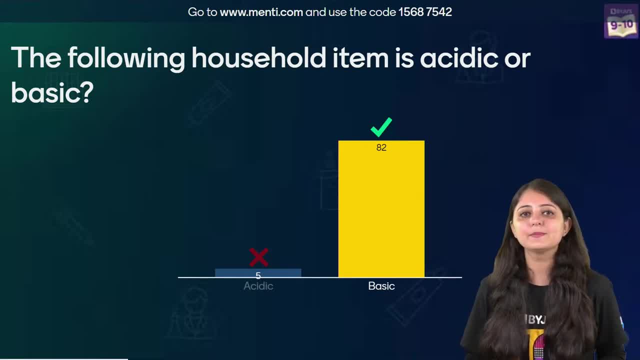 And I can see series of thumbs up coming my way. I think this is going to be a super amazing chat box here. 5 seconds. 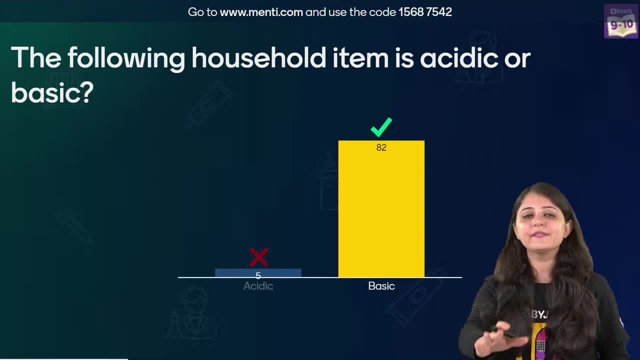 5 seconds. Priyanka is saying, ma'am, I will solve all the questions in 5 seconds. You just give me 5 seconds. 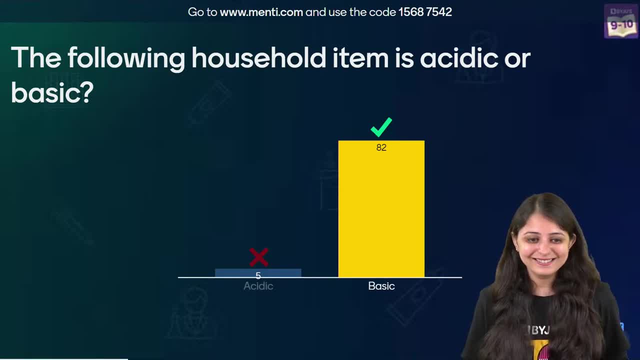 0.7 as in Rajesh said, 0.7 seconds in answer. Okay. Anub wants to see the leaderboard. We will show the leaderboard. It's going to be a really interesting session. We will build a little suspense and definitely we will show the leaderboard. 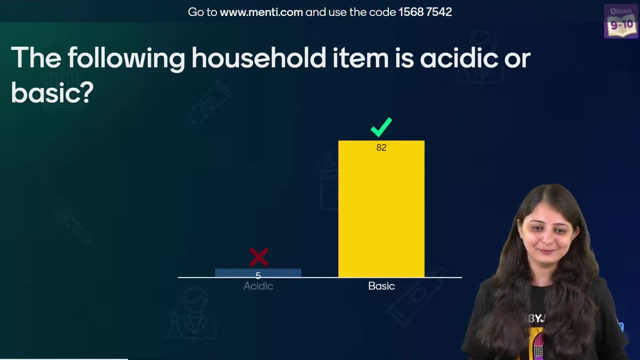 But yes, as soon as we will show the leaderboard, I want all of you to post your rank. Good. Alright. Yes. So, 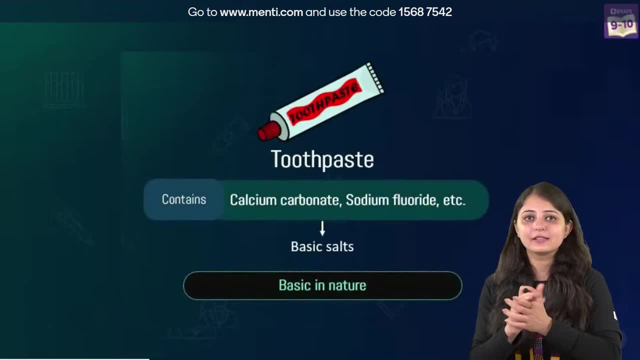 Toothpaste, it contains sodium fluoride, NAF. But sodium fluoride is also present in pesticides, right, poison. You will get sodium fluoride in a lot of items. 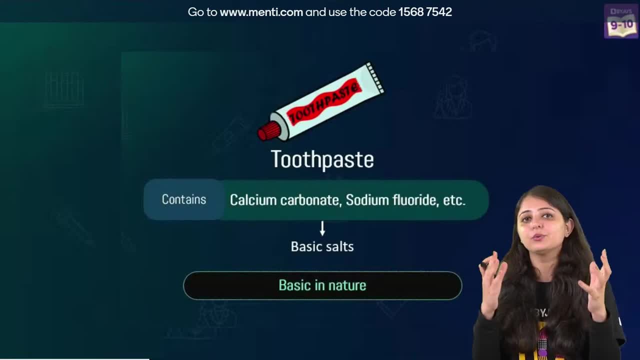 But why exactly are we using a toothpaste? When we eat something, the food is broken down into smaller substances, right. So, the bacteria that's present in our mouth, actually it's releasing acid. 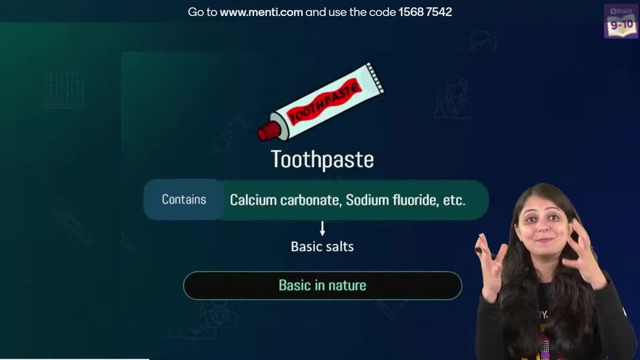 And to neutralize that, we are using a toothpaste. So, toothpaste is basic in nature. So, now we know, the first one, lemon contains an acid. 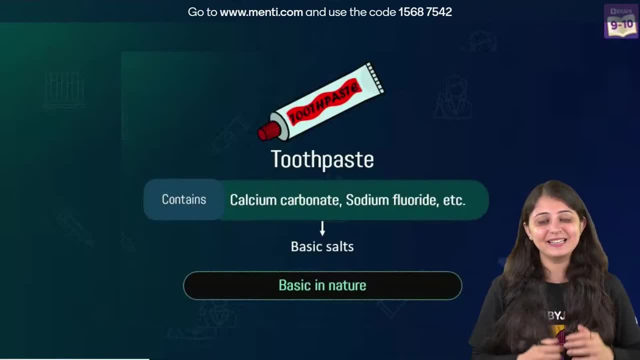 Acidic acid, sorry, citric acid. So, that was acidic in nature. So, lemon is acidic. We know toothpaste is basic. Yes. Great. Yes, sodium fluoride. Absolutely right. Yes, yes, lemon contains citric acid. Good. Awesome. Chalo. Let's move on to the next question. 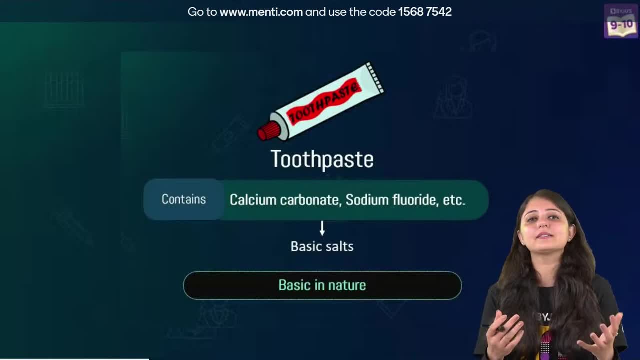 Absolutely right. See, you are understanding the concept of neutralization beforehand only. Though we will be covering that topic in detail. But you have also studied in class 7th. Okay. Let's move on to the next question. Question number 3. 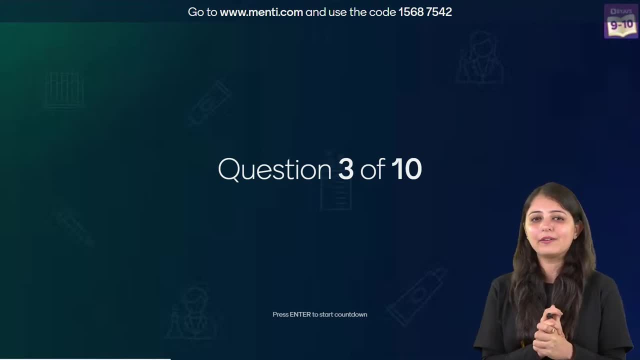 Innovative. 26 has given us an innovative idea that leaderboard would come after 5 questions. Okay. Done. Question number 3. On your screens. Ta-da. Now. 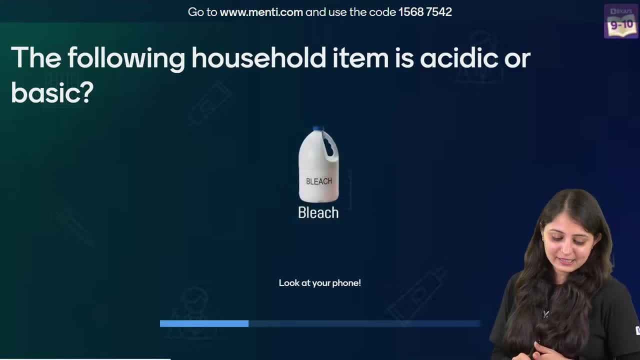 Let's see what the question is. What's the household item now? Okay. Bleach. 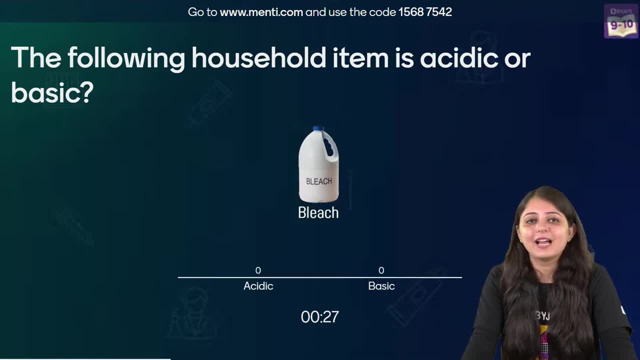 You might get confused with this one. Bleach. Is it acidic? Is it basic? What is it? By the way, where is it being used? You can think about that also. Socho. Socho. You have 15 seconds left. Hey, no answers in the chat box. 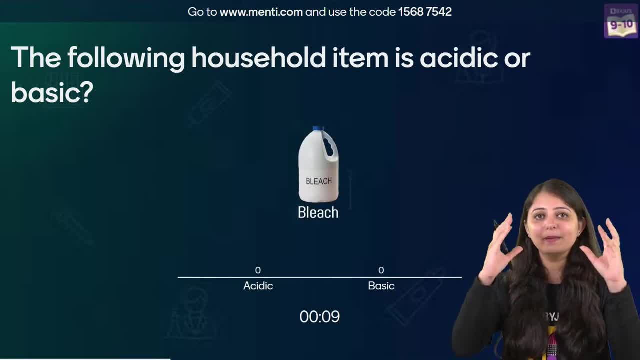 Rules follow. You just have to mention the time in which you've answered. Or maybe give me a thumbs up once you're done. Last 5 seconds. 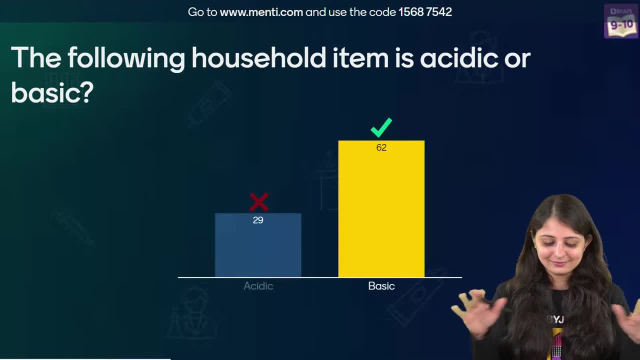 3, 2, 1. And done. Hey, this is a question where some of you got confused. 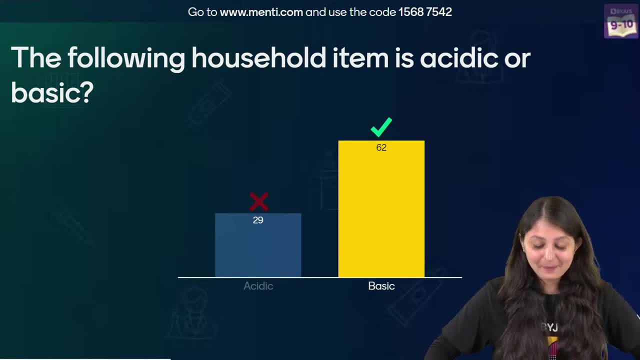 Okay. 62 students have voted for basic 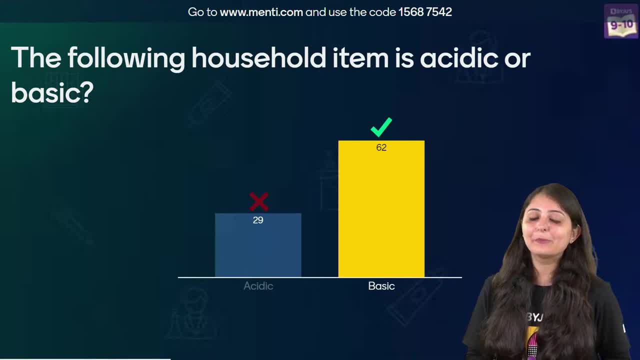 A very high number, I would say, have also voted for acidic. So, it's a very good thing that this has come up. Because now this way you'll actually understand what is the nature of bleach. What is it? Acidic is basic and why? 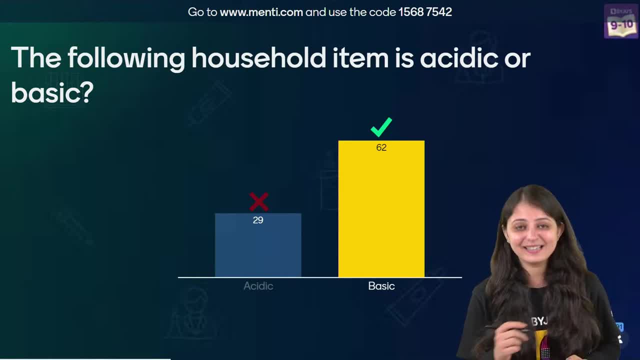 Where is it being used? So, yes, the correct answer was basic. So, there you go. 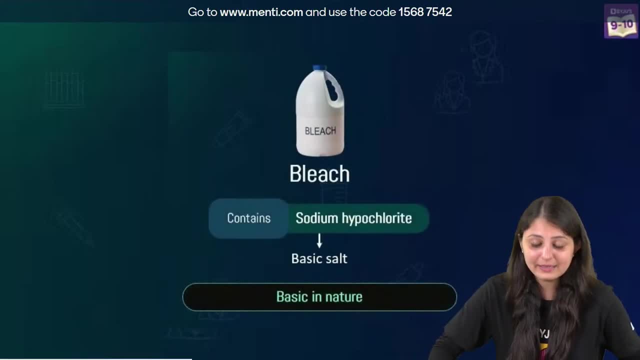 Bleach. It contains sodium hypochlorite. Sodium hypochlorite is actually NaOCl. 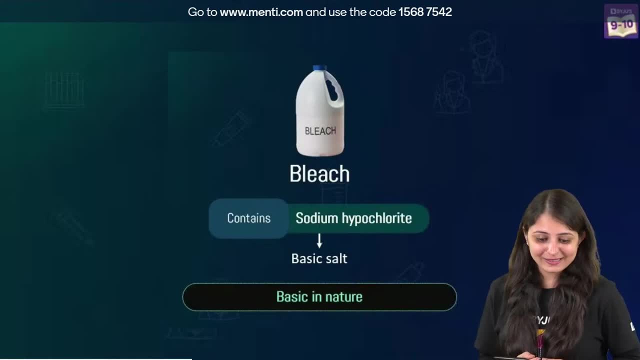 Now, this is completely a basic salt that you can see over there. Yes, absolutely 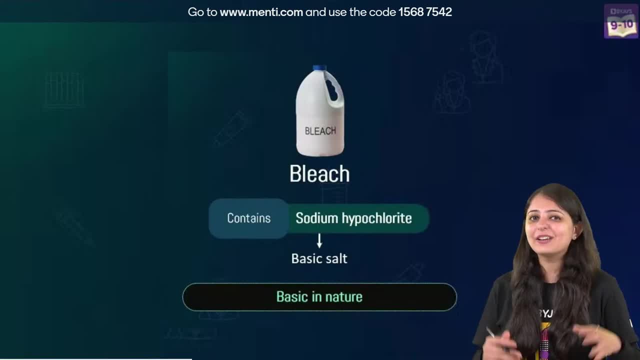 right. So, bleach is basically being used to clean and remove stains. 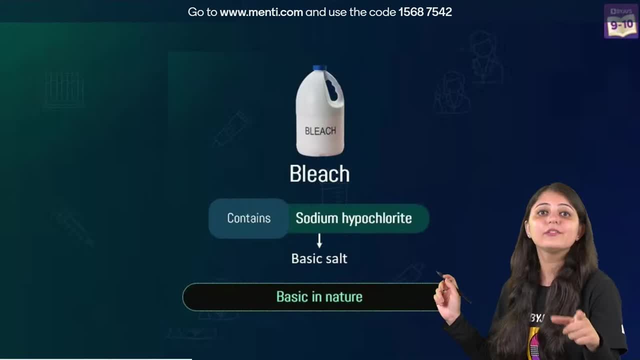 Okay. It's not bleaching powder. Don't get confused with bleaching powder. Bleaching powder, is calcium oxychloride. CaOCl2. We'll come to that also. But this is bleach. Yes, Manas, we're good at removing stains. Absolutely right. Correct. Saif Safdar is saying, ma'am, I did acid but I did in 5 seconds. 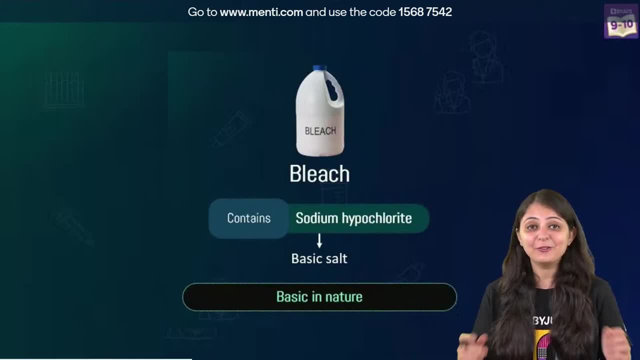 No, not like that. You have to be quick but you have to be accurate also. 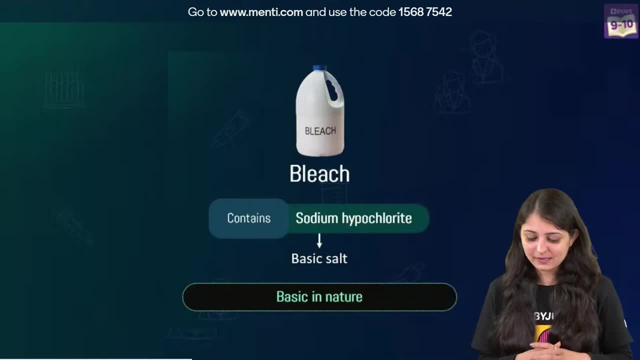 Hey, Mani, it's okay but just start answering now because it's going to be super amazing, right? Okay. Question number 4. 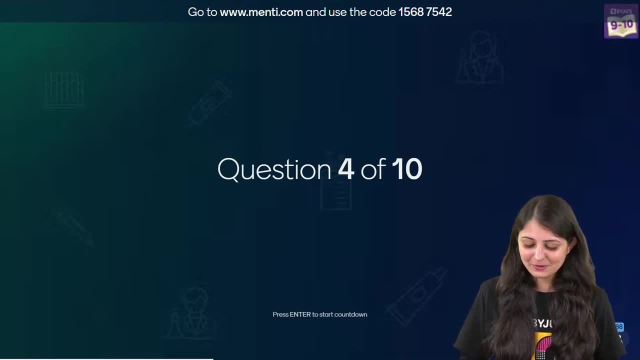 And let's see. This is going to be really important question actually. Question number 4. 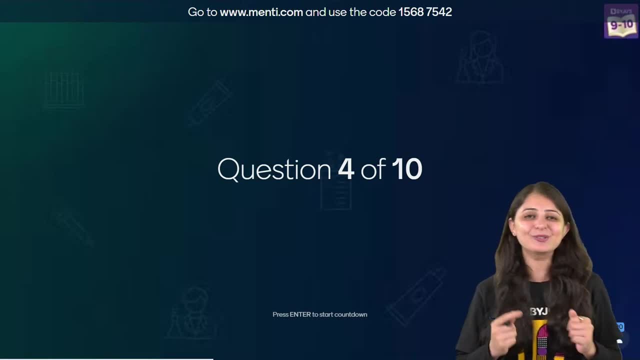 I'm sure half of you are just making random guesses. What household item is going to come next? Hey, Rohan, that's awesome. Absolutely. 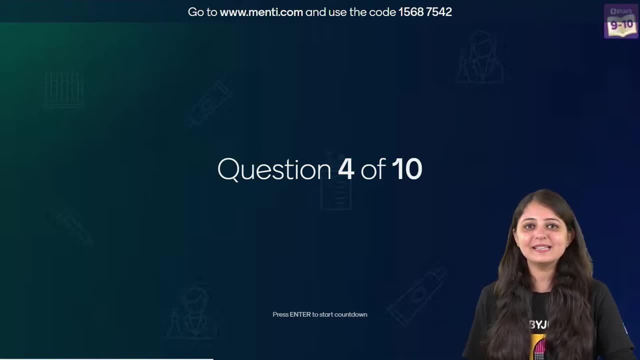 Chalo. Question number 4. Let's attack this question as quickly as possible. 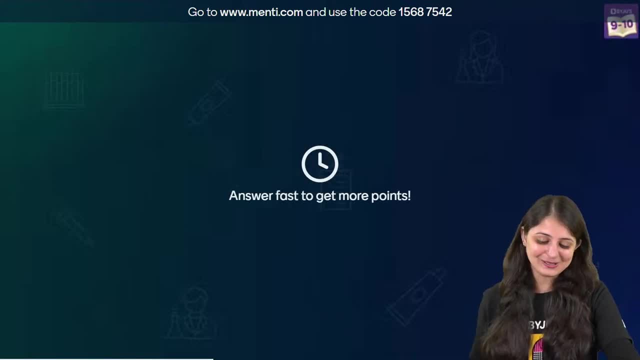 But let's not forget to be correct also, to be accurate also. 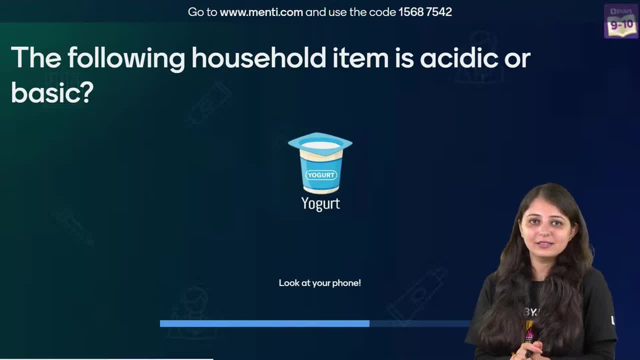 The next wonderful item that we have is yogurt. 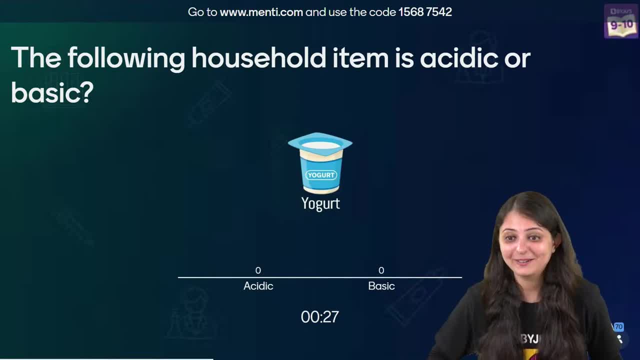 I think you might get confused. You might not get confused. Let's see. Let's see. You've got good 30 seconds, by the way. Hey, Jyoti, I hope you're getting all the answers right. 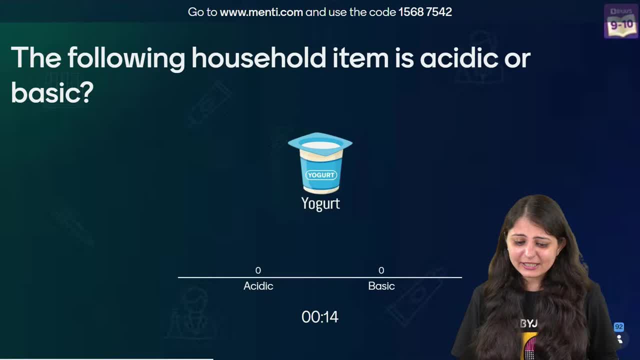 So, is yogurt acidic in nature? Is it basic in nature? Yes. Let's see. Let's see. We have last 5 seconds. This is awesome. Great, guys. 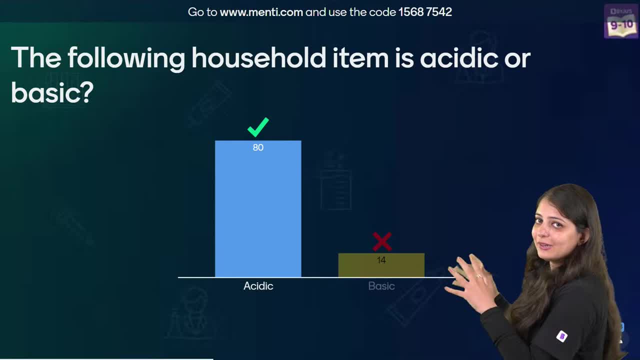 80% of you, like 80 students, not 80%, 80 of you have voted for acidic. 14 are saying it's basic. 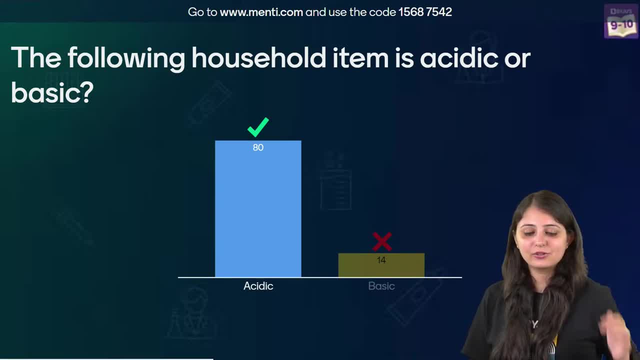 Nikita has already mentioned the acid also. That's present. 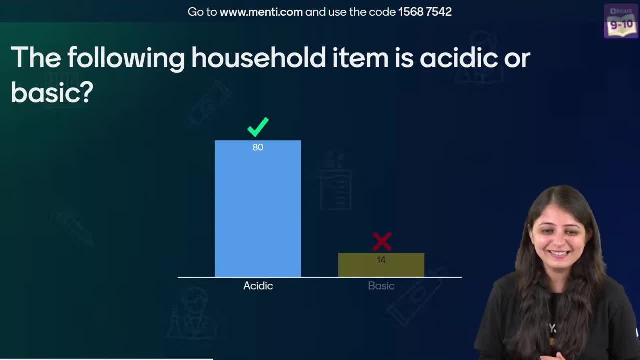 Yes, Anushka, you're a bit late, but it's okay. Quickly join in. Yes, Manasvi, absolutely right. Innovative 26, I want to know your name now. 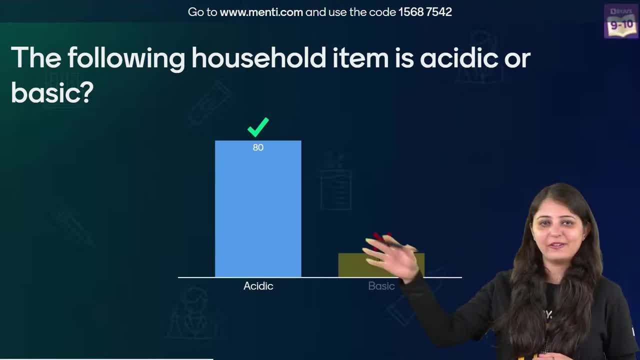 I don't know how many zeros you've put. Zero point, I don't know. Infinite zeros and then one second that you've answered the question. 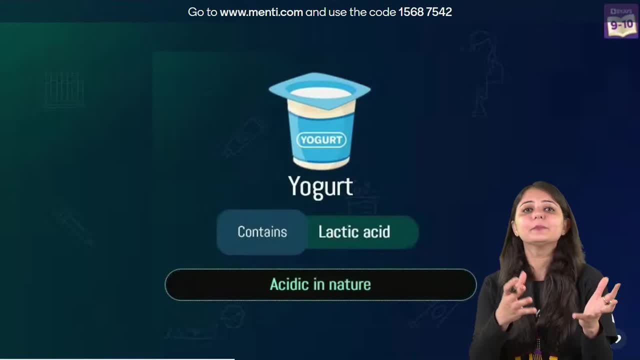 Great. So, yes. You know, it's like the scented milk, yogurt, right? It's semi-fluid. 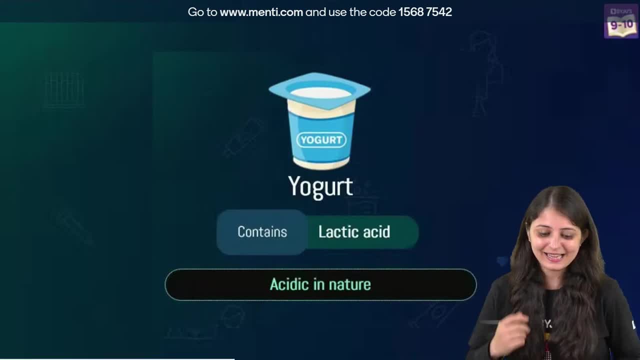 Which acid is present? You people have already mentioned it. It's lactic acid. So, yes, this is absolutely right. Good. Yes, lactic acid is also present in milk. True. 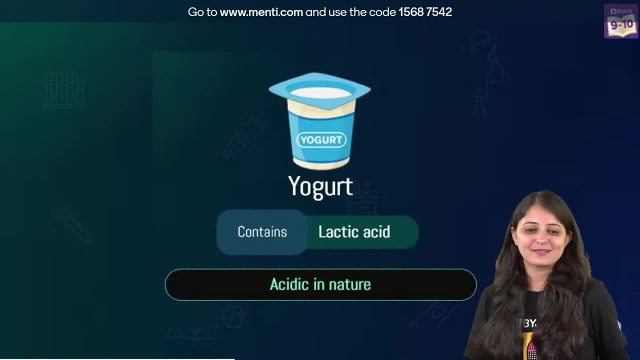 In sweat also, by the way. In our sweat also, lactic acid is present. Oh, your friend is lactose intolerant. Correct. Correct. 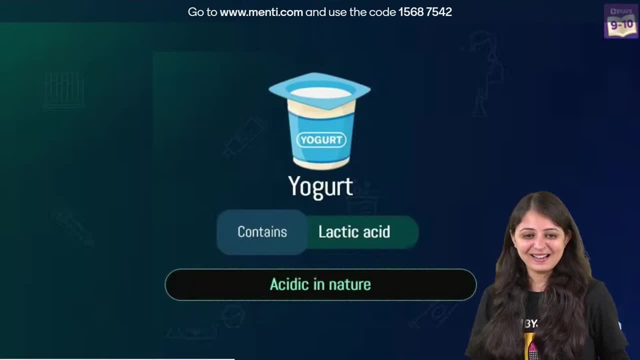 All right. Your name starts with letter A. Okay. Great, great, great. 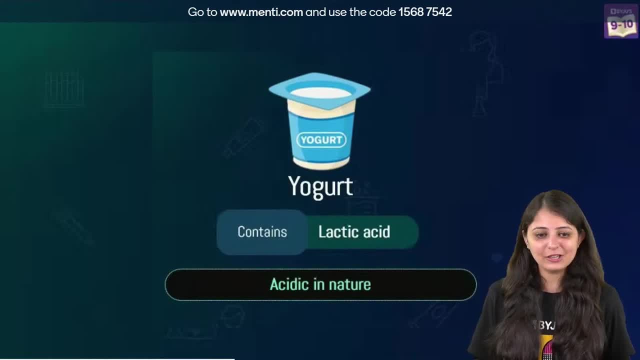 Good going so far. It's fun to see how quickly you people are answering. And do you know the best part that is happening over here is before the time gets over in some of the questions, 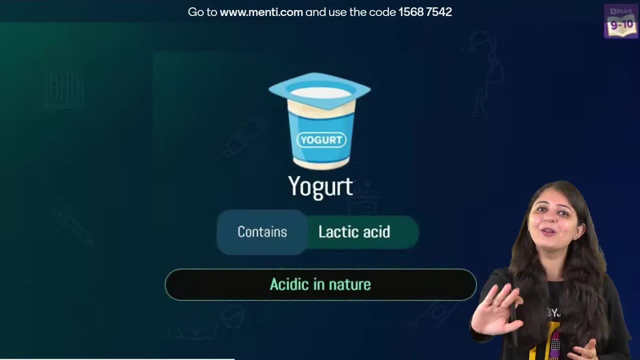 from many meters, the instruction is coming that all of you voted already. That's great. All right. 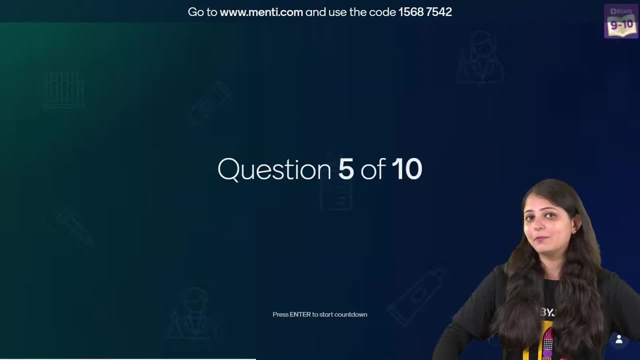 Let's move on to the next question. Okay, this question number five is very important. Super important question. I'll tell you why. Because many of you are asking me, Ma'am, when will the leaderboard come? So, to show the leaderboard, after this, we'll reveal what the leaderboard is. 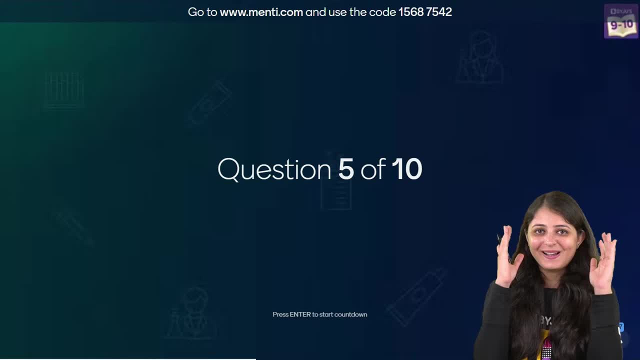 So, anything can change after this question. I want all of you to be really focused. Some interesting household item is going to come up. Pay attention. Pay attention well. 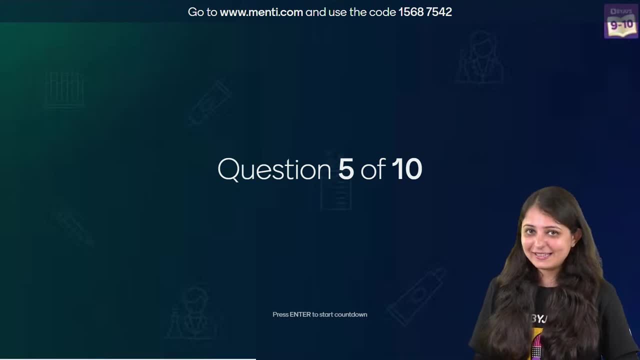 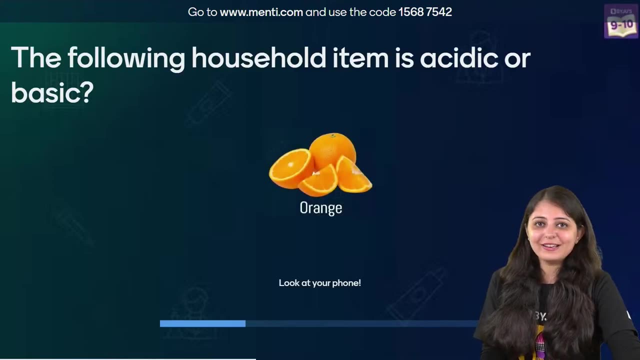 And next household item that you have to decide whether the nature is acidic or basic is orange. Come on, let me answer in a second. Quickly. Answer this one with lightning speed. 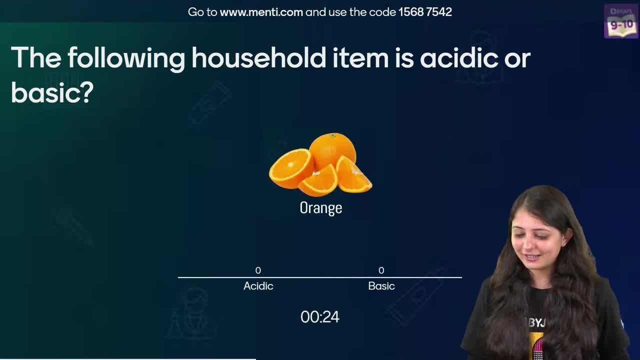 This is, this is like I think I should, I can take it for granted that it will come. Can I take it for granted? Tell me, tell me, tell me. Quickly. Hey, 99 of you are there. Let's see. How, how quickly we can make it a hundred. Hey, awesome. 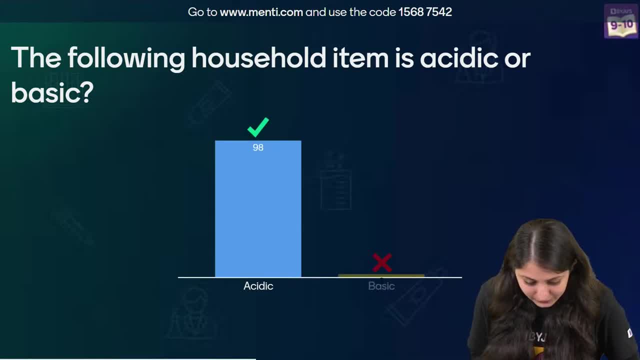 100 kids are out there attempting the questions. Out of which 98 of you got the answer right. This is super amazing. 98 of you got it right. Both of you have scored basic marks. 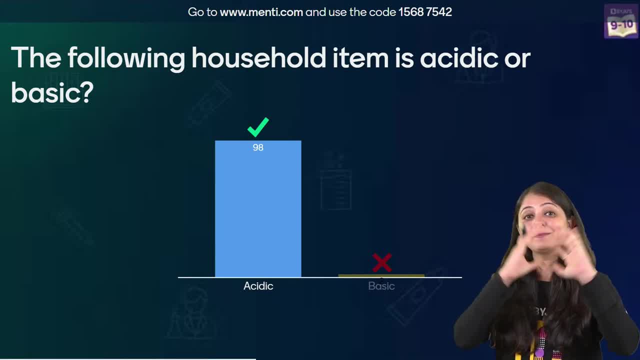 Okay, if you've actually, if you were focused enough, maybe towards the beginning, when we were discussing about lemon containing citric acid, we came across this also. 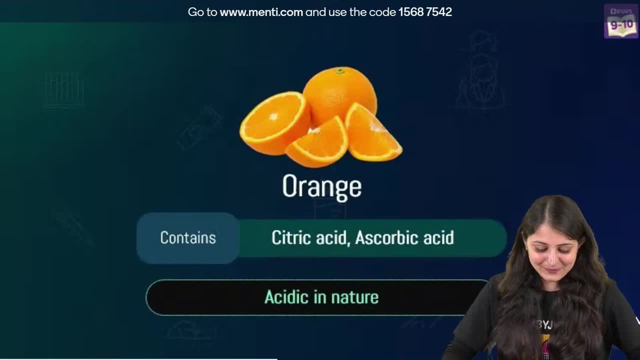 Yes, I told you, you know, all citrus fruits, they contain citric acid. So, in orange, you will also get citric acid, which is by the way, also used as a preservative 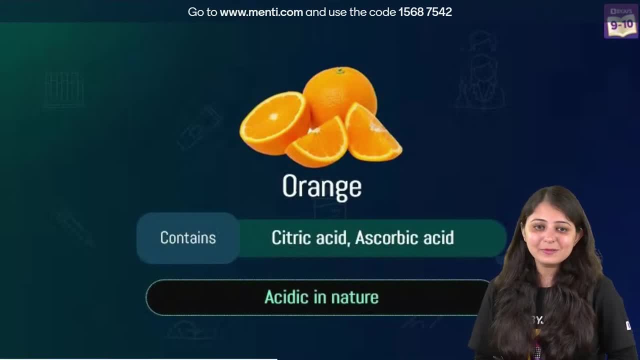 and ascorbic acid will also be available. You must have heard about vitamin C, right? Okay, what are the diseases caused by vitamin C deficiency? Quickly, let me know. I did it in grade 6. Long back. No one says, yes, ma'am, you told. See, I'm giving you hints here and there already. Scurvy. Scurvy. Great. 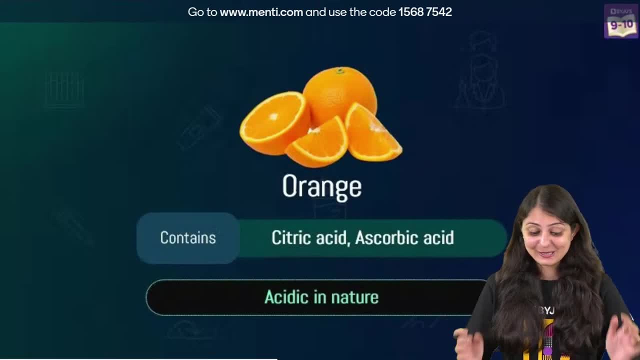 Okay, it's time to show you the leaderboard. Since many of you, in fact, I should say all of you, are showing a wonderful performance. 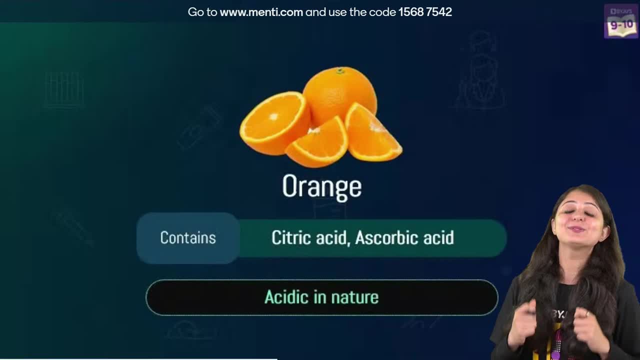 Means, you are showing a very impressive performance. Even I am super curious this time to see the leaderboard. 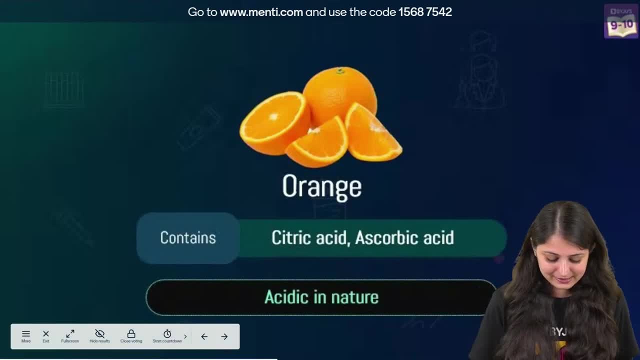 Okay, let's go. Fingers crossed. 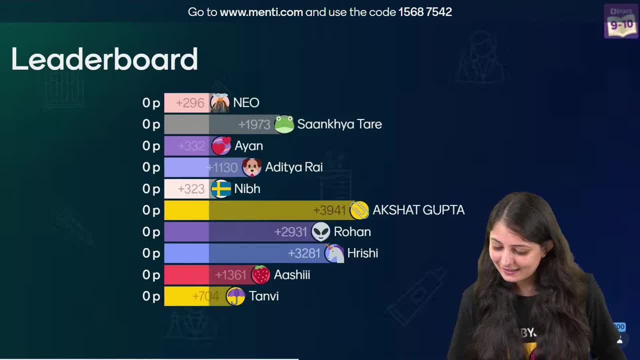 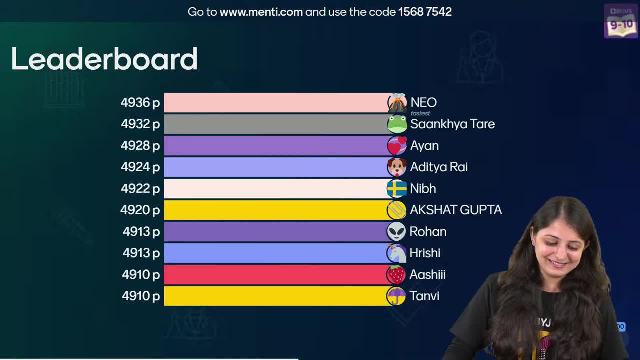 Let's load the leaderboard. And let's see who is there at the top. Who are? Top 10 chemists, I would say. Okay, so the fastest is Neo. 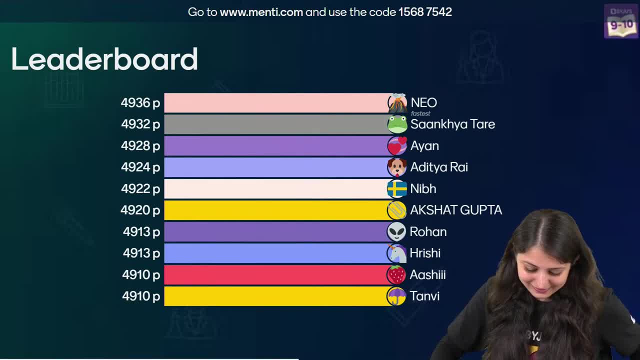 And then we've got Sankhya, Ayaan, Aditharay, Neb, Akshat, Rohan, Rishi, Ashi, Tanvi. Well done, guys. 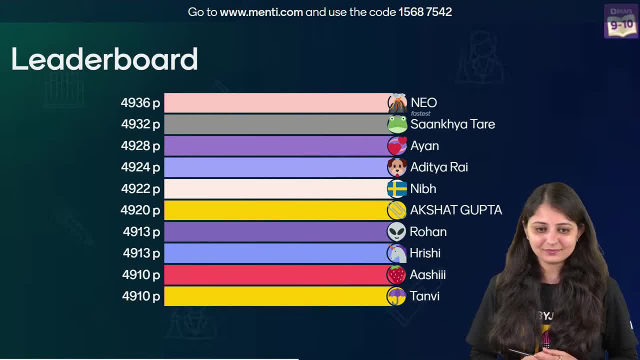 Now, it's your time to quickly let me know your rank. See, out of 100 students, if 98 of you are getting it right, you already are, you all are geniuses. Already. Super impressive performance you are showing. I just want to know your rank right now. 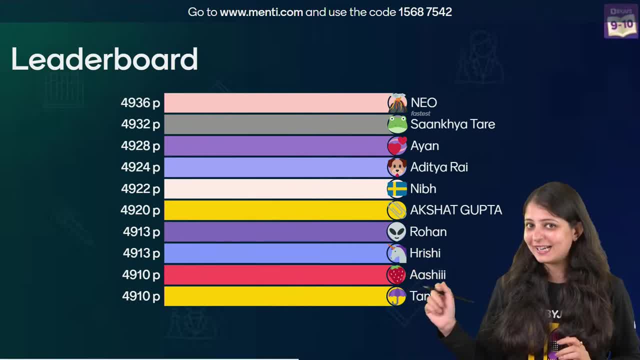 Because the next time when I show you the leaderboard, I want to see at that point of time, whether you have improved your rank or not. So, it could be any number. Doesn't matter. 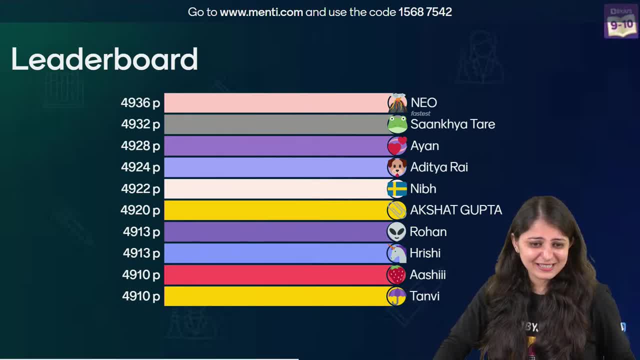 34, 27th, 52nd, 76th, 23rd, 70th, 45th, 12th, 16th, 50th, 28th, 37th. Hey, after 37, why have you made so many angry faces? Why have you made so many angry faces? It's a good rank. 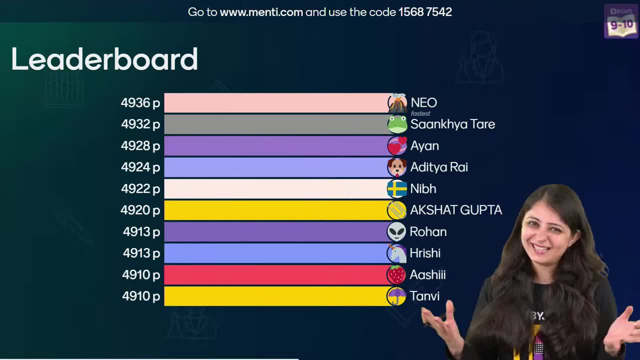 7th, 77th, 85th, you joined late. That's okay. But, but, but, we are just done with half of the session. 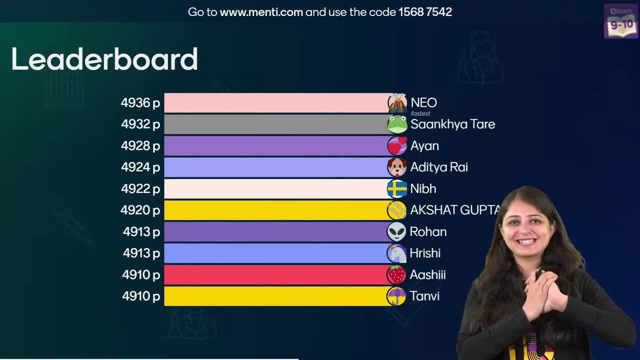 We have 5 more wonderful questions. So, yes, keep thinking. Keep your mind stimulated. 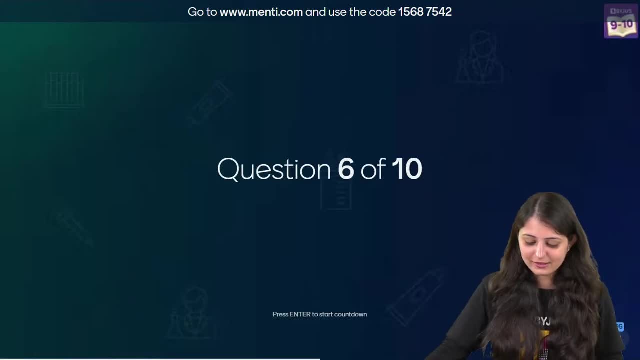 And on this positive note, let's move on to question number 6. 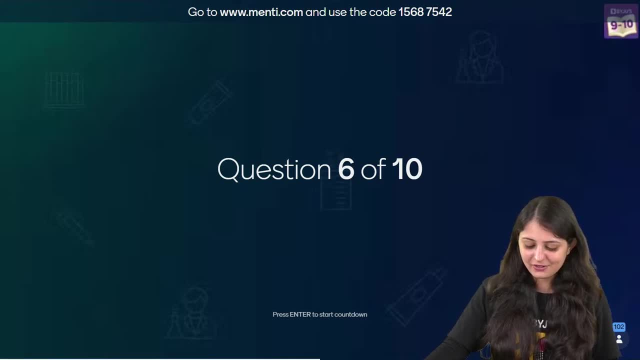 And yes, we have a perfect 100. In fact, 101, 103 students with us. 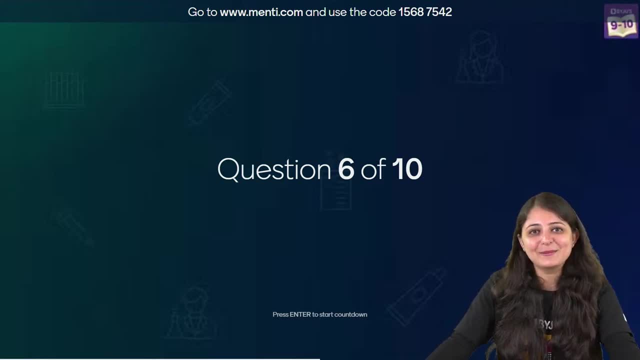 So, let's see what the next household item is going to be. It's going to be fun. Let's see what the next household item is going to be. Let's see. 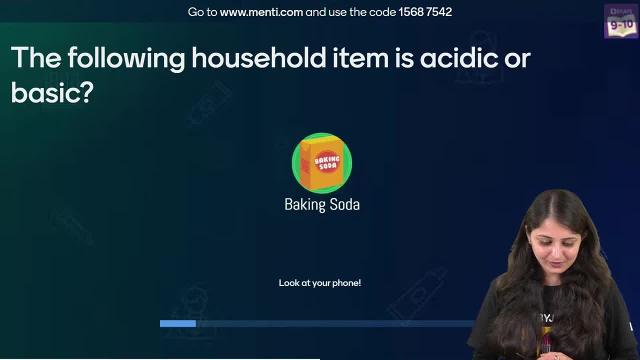 So, question number 6 on your screens now. Baking soda. 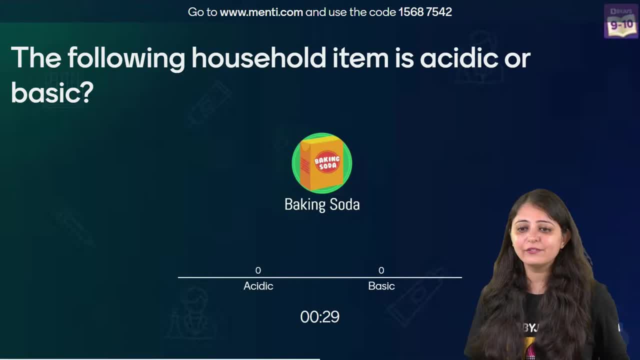 Hey, we've used baking soda so many times. Tell us the answer to this quickly. Is it acidic or basic? I think this one's really simple. Quickly, you can let me know. No, no, not here. Not here in the chat box. You've got it. No, no, not here. Not here in the chat box. 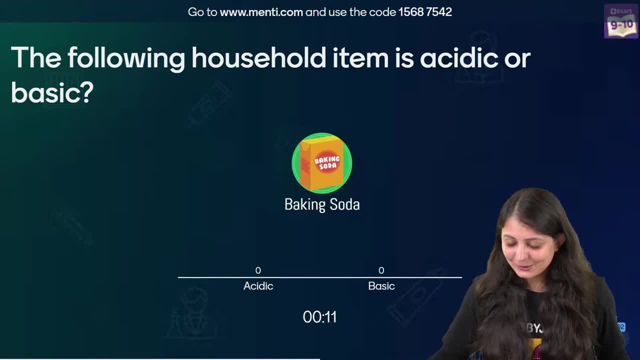 You've got 10 more seconds. Though I am kind of super confident because we've been studying baking soda for a long time. Acidic or basic? Let's see how many of you are going to get this one right. Well done. 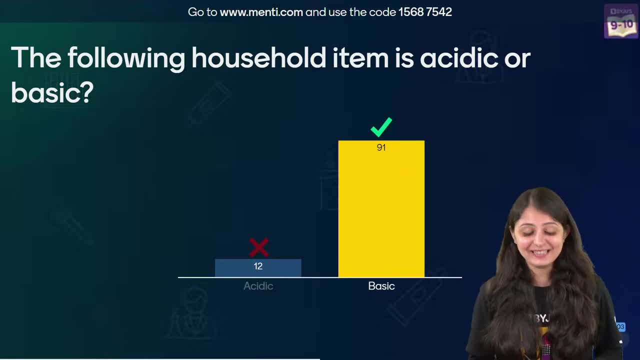 Well, well done. 91 of you got the answer right that it's basic in nature. 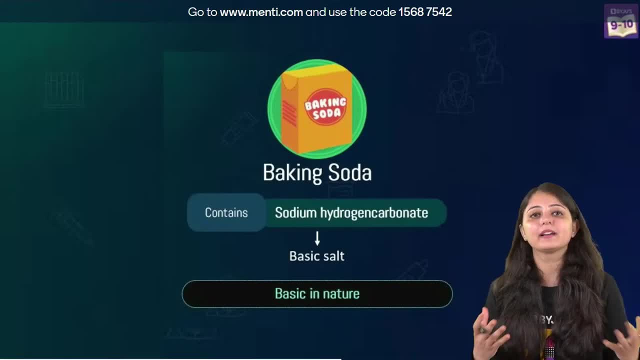 Absolutely right. So, baking soda is sodium bicarbonate. That's sodium hydrogen carbonate. It's a basic salt. You know, it's also being used to make baking powder. We'll study about baking powder. Don't worry. 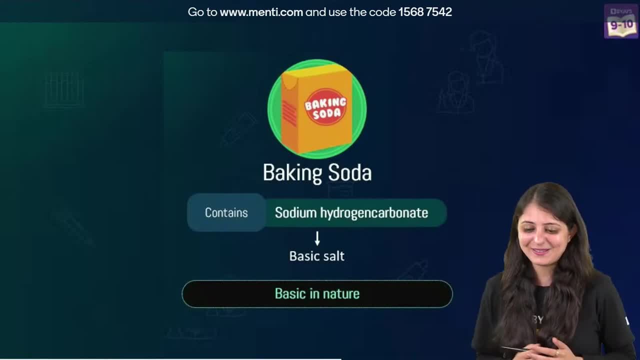 We'll tell you what's the difference between baking soda and baking powder. Don't worry about that. And also, it's being used as an antacid. It's also used in soda acid fire extinguishers. So many places, so many substances are actually containing baking soda. 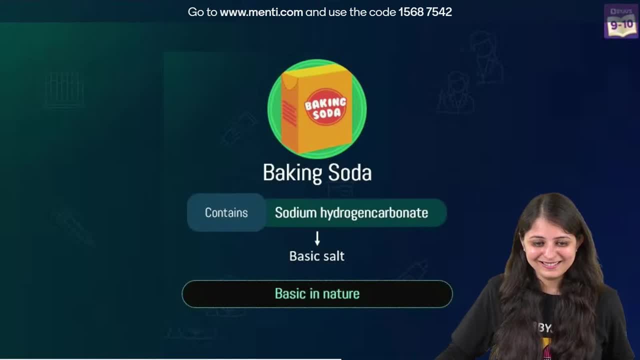 Hey, Niva. Noted. 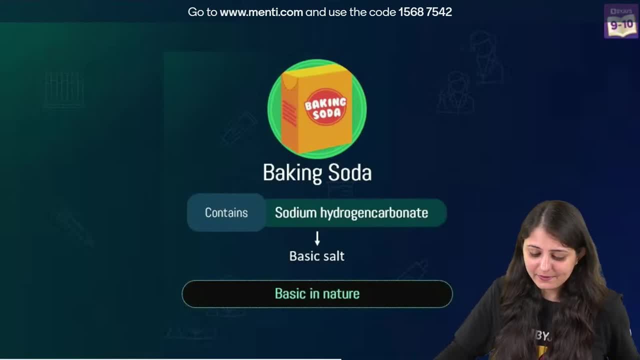 Hey, Prashantsa. The code is 15687542. Quickly join in. We are still left with a lot of questions. 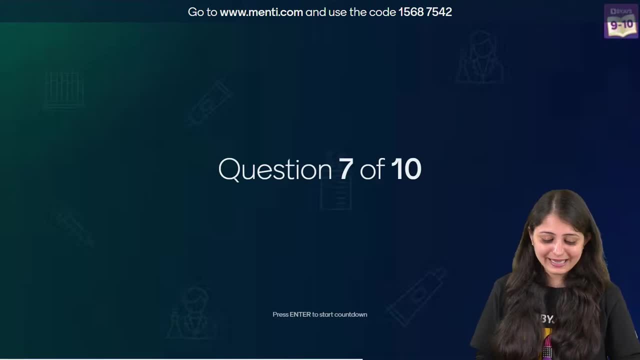 And let's move on to the next one now. Question number 7. Four more questions to go, guys. Basic. Yes. Manjunath is saying, next question please. So, let's listen to Manjunath. And let's load the next question. Some of you are just having some food items there. Okay. Vinegar. Hey, okay. 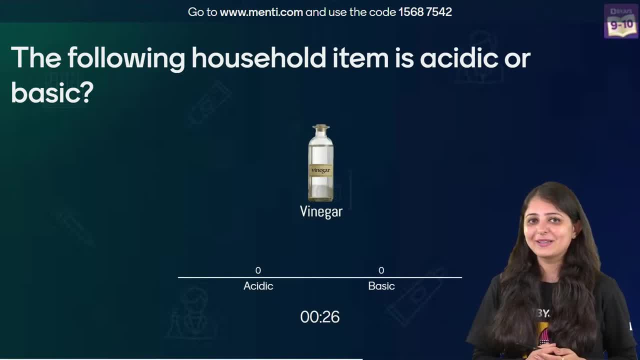 So, I was also confused. I was having this bottle of vinegar with me. And I was asking you on the telegram. Is it acidic? Is it basic? Is it containing an acid or a base? So, you can help me out now. 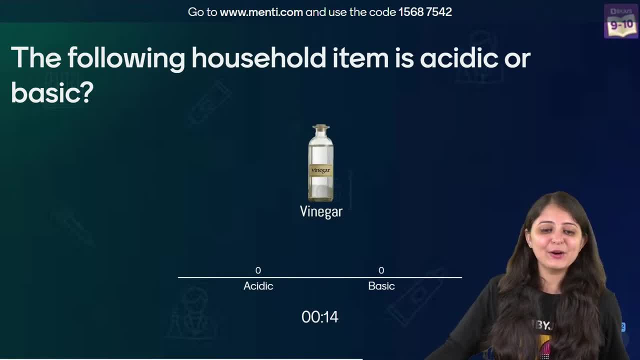 I don't know. You people have to help me. I'm counting on you. Quickly answer. 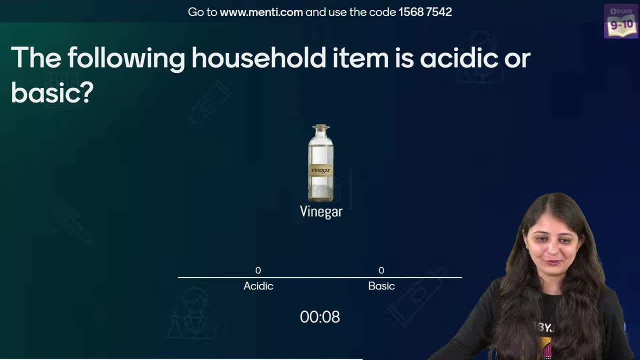 So, if all of you will get this one right, then only I'll go with that vote. You're answering very quickly. Good to know that. Okay. 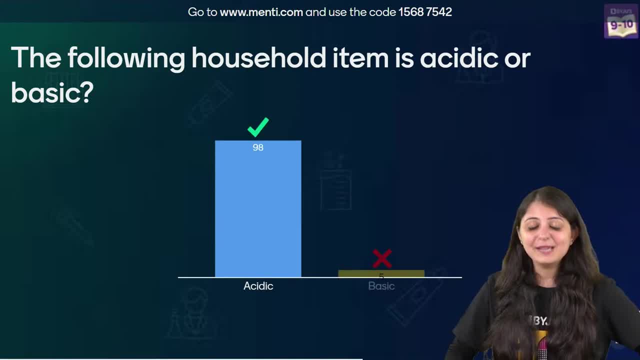 98 of you got the answer right. I mean amazing. I'll, you know, in some time, I'll be short of all good adjectives for all of you. Because you're giving such a good performance today. 98 students have voted for acidic. And that is the correct answer. Great. So, yes. Vinegar contains. Acidic. Acid. 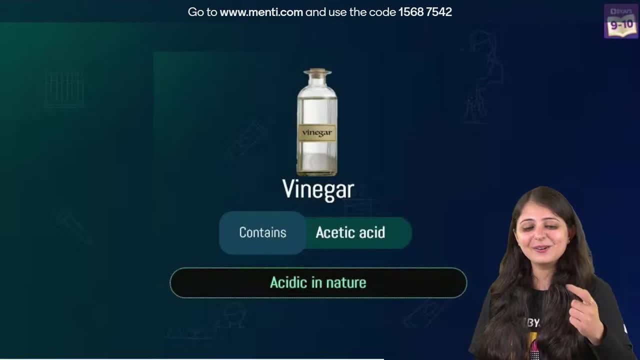 You people are right. Some are revealing answers here. No problem. It's okay. 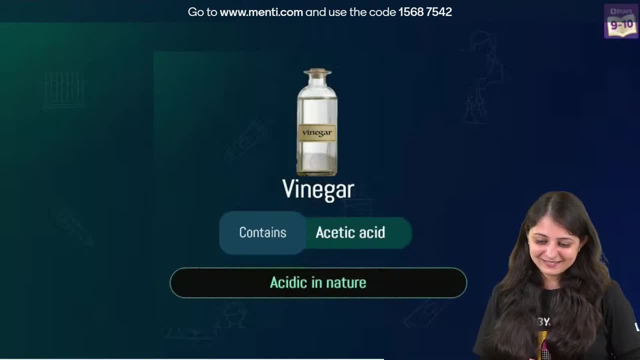 Just give me a thumbs up once you're done. Yes. 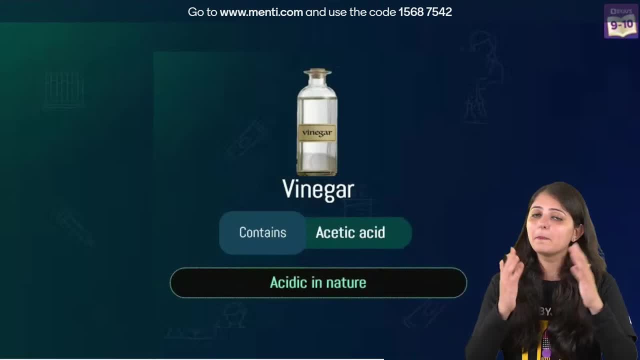 So, acetic acid, by the way, it's also present in medicines, paints. You'll get acetic acid in a lot of items. I'm not ignoring anyone. All of you are here. 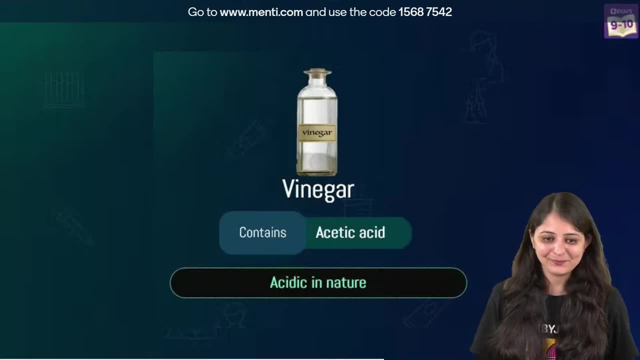 And all of you are enjoying this. And that's the most important thing. 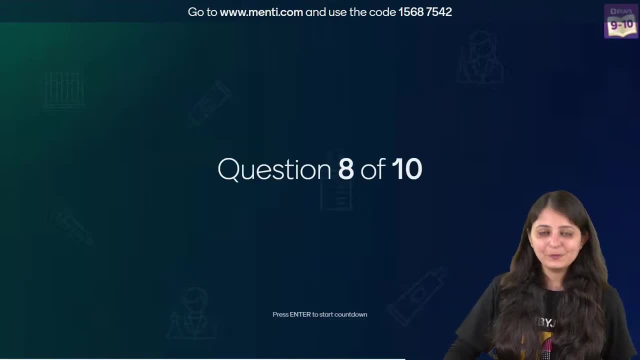 Let's move on to the next question now. Question number eight. 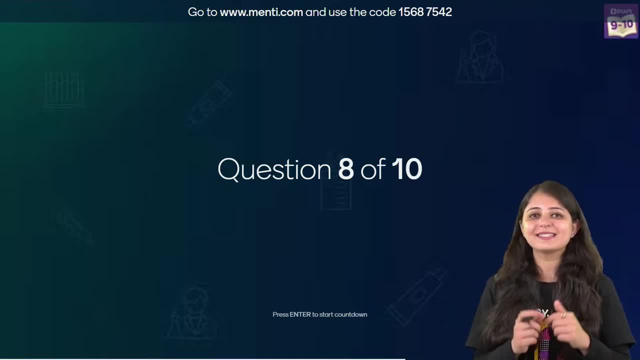 You know, before I reveal what the question is, what's interesting is that which household item will come next? Divyansh, let this be the menti first. Ravi, Chandran, not so angry. We have to give answers. Now, enough. Give the menti an answer. Just give a thumbs up here. Jitin, is it seventh grade or attempting grade? 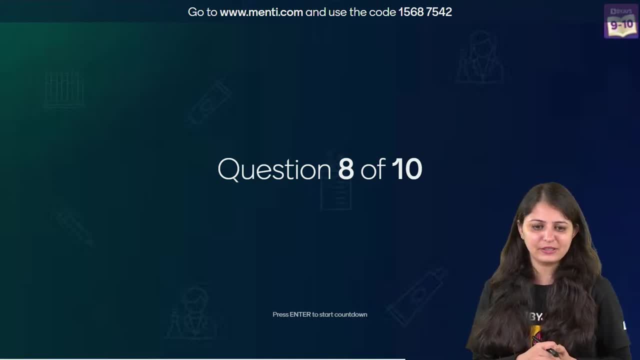 Acid is in seventh grade and attempting this, yes? Acid basis is there in seventh grade as well. You definitely can attempt these questions. Okay. All right. 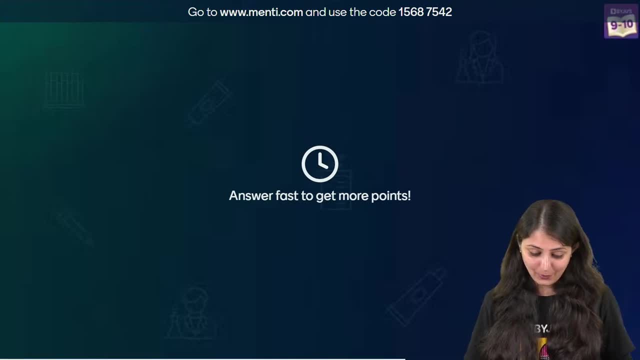 So, question number eight on your screen now. Let's see what's the next one. 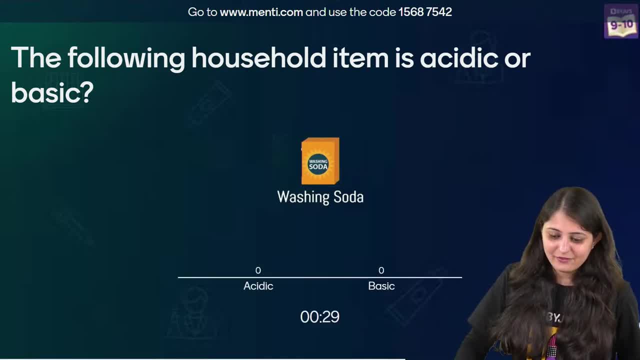 Washing soda. Okay. 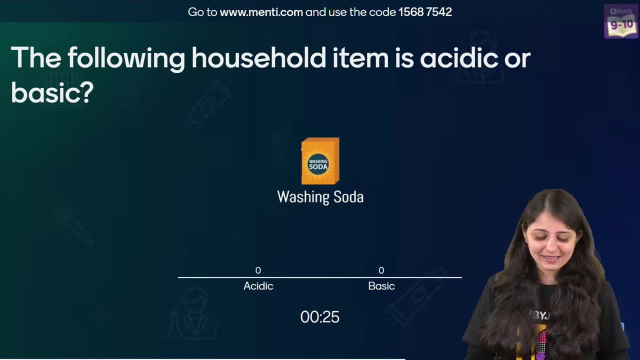 Where is washing soda used? Is it acidic? Is it basic? Currently, you just have to decide the nature. You might have heard about washing soda. 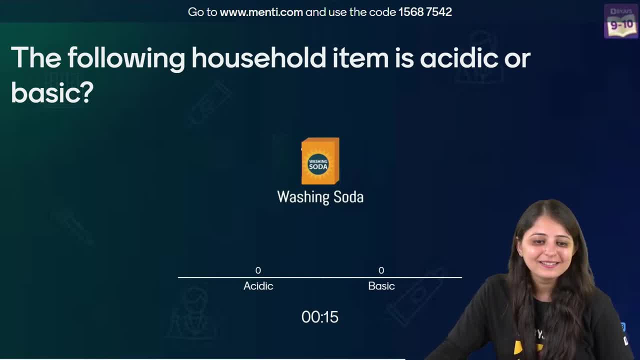 In fact, if I'll tell you the use, you'll understand in a second. 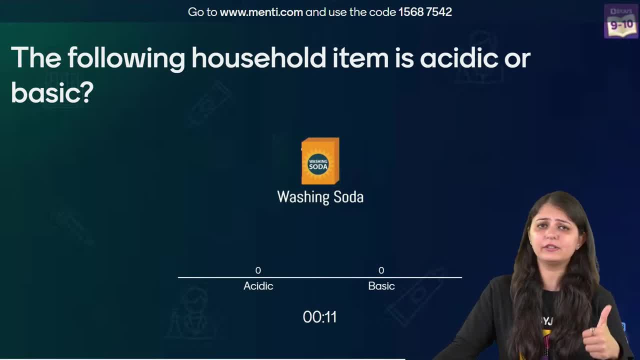 Gaurav Vagela has given me a thumbs up. His thumbs up came up very quickly. 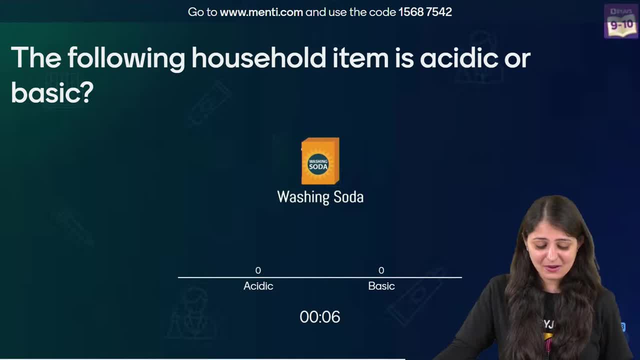 Muskaan, Himani, Nibha, Prem. Great, man. I mean, you all are amazing. All right. Time's up. Ninety-nine. Almost a hundred. 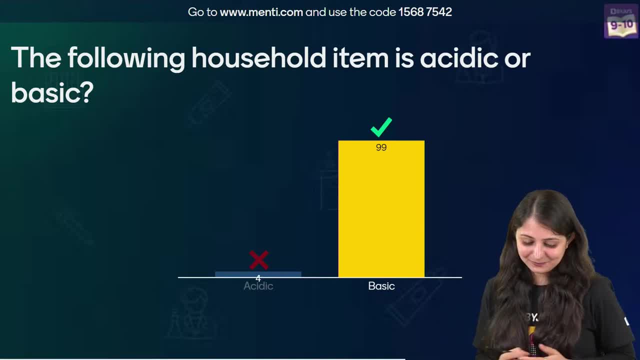 You know, I'm just hoping that we'll cross a hundred in any question. 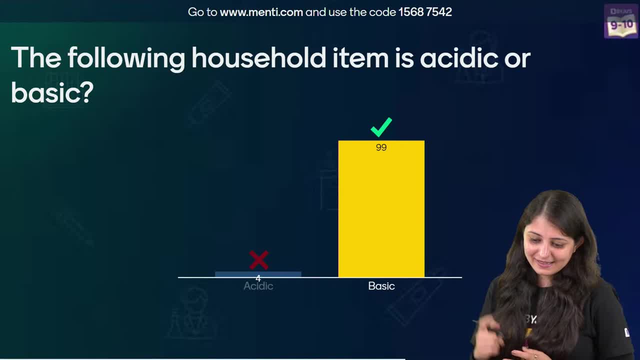 Ninety-nine of you got this one right. That it's basic. 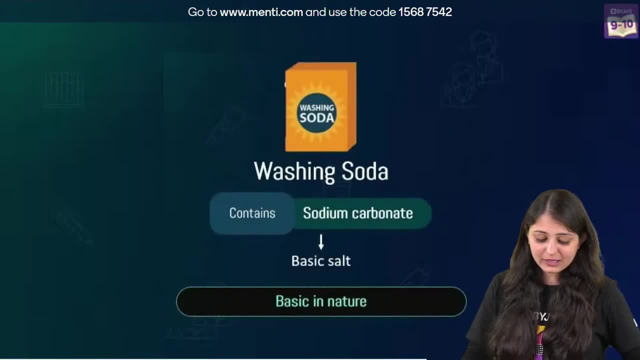 And you people are absolutely right. So, washing soda is sodium carbonate. It's also a basic salt. So, yes, you people are right. 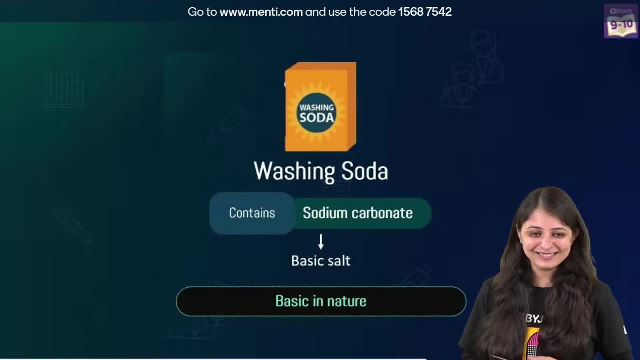 You know, it's being used for cleaning clothes. Good. 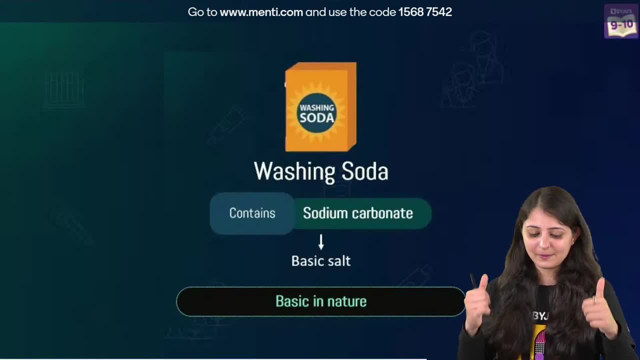 Awesome. I can see loads of thumbs up. Loads and loads of thumbs up out there. 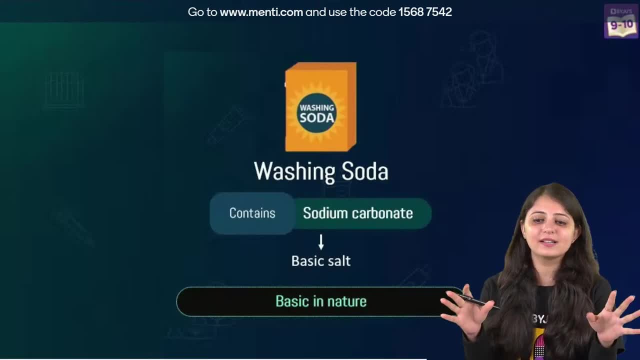 Innovative26 is saying, I've answered the question infinitely fast. So, you people can see yours. Yes, Himani. 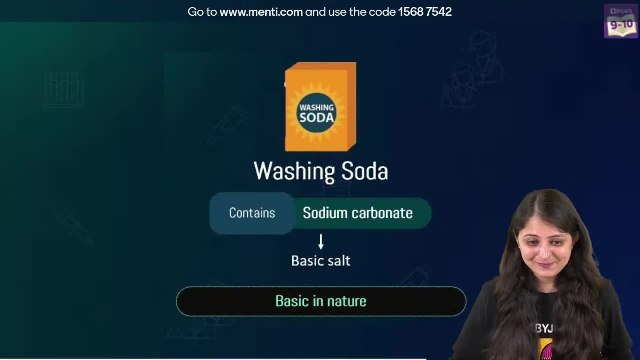 Correct. Detergent. Yes. Sodium carbonate. Yes. Absolutely right. Yes. You people are right. In fact, and it's also used in glass industry. Paper. Paper industry. There also. Correct. Yes. Absolutely. Soap maybe. Detergents maybe. Yes. Yes. 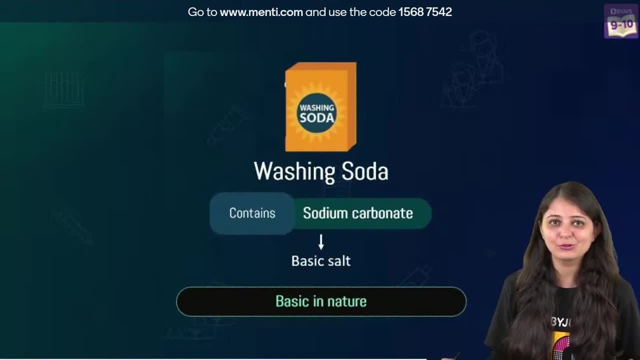 Sankhya wants to see the leaderboard. Not so soon. We are left with one more question. I know you people are super excited to know who is leading the leaderboard. Scoreboard. How is it looking now? 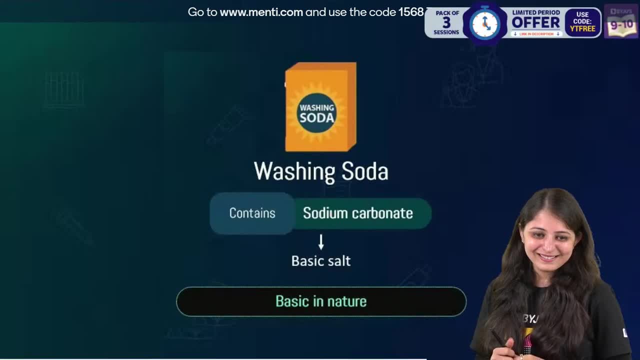 Okay. Question number 9. 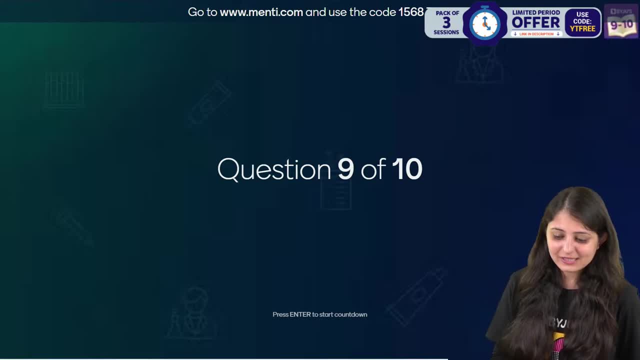 So, we are left with two more questions. Question 9 and then question 10 and then the leaderboard will be right in front of you. 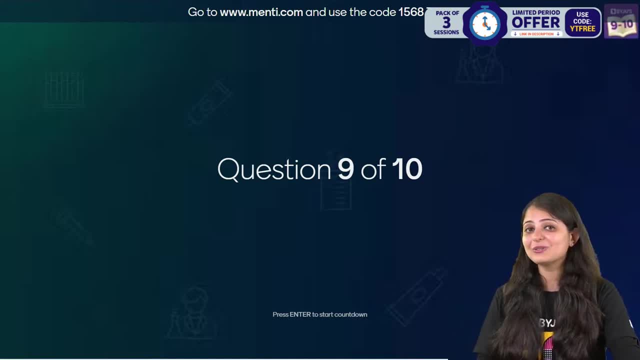 Let's load question number 9. Two more questions to go, guys. So, buck up. Be pepped up. Be charged up. Two more household items you have to identify and that's it. And there you go. Then you would know a lot about chemistry around you. Divyansh is saying, I like your class because of English. Okay. Okay. 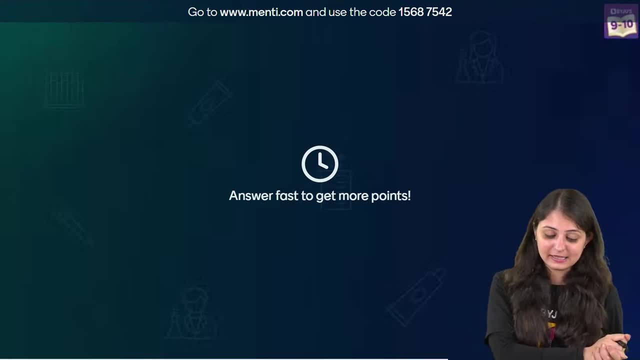 Question number 9 on your screens now. 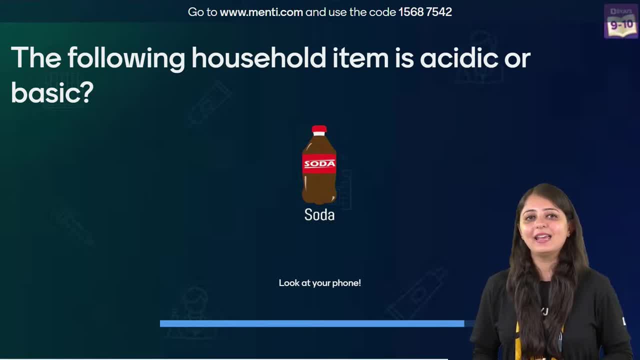 Hey, everyone's favorite. Everyone's favorite. Soda. Is it acidic? Is it basic? I think we have to find out the answer, out of interest. 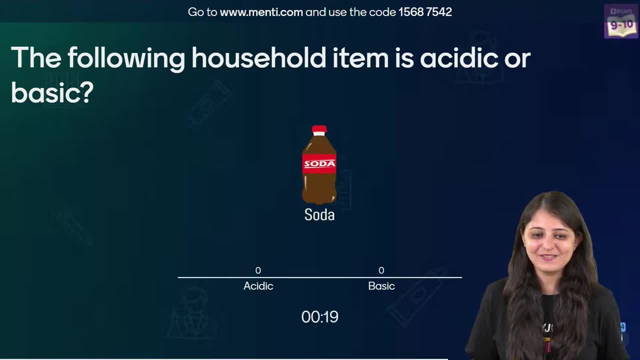 You should know this definitely. Yes, Sathyam? 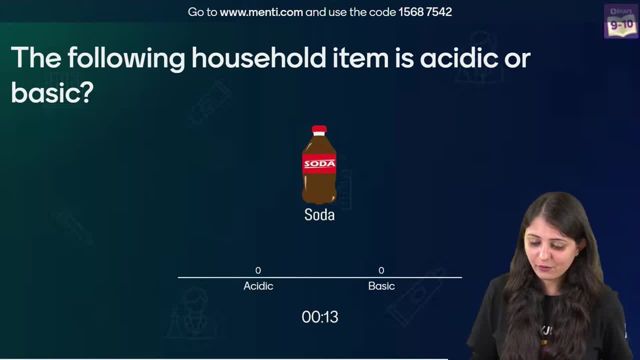 The code is 15687542. 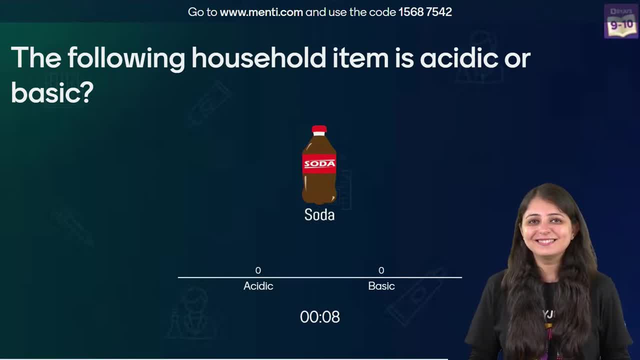 Quickly answer this one. We have around 5 seconds left. 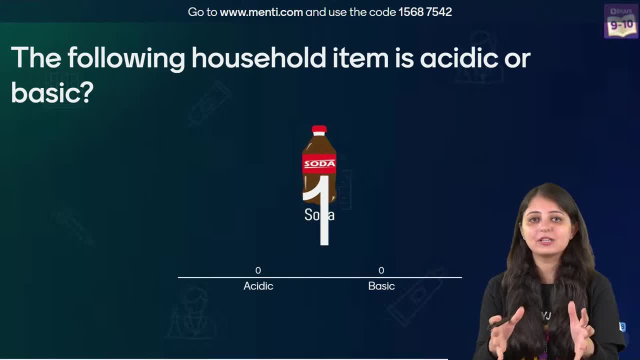 And in fact, if you don't know the answer, it's a good time to understand what's present in soda. So okay. We've got a mix here. 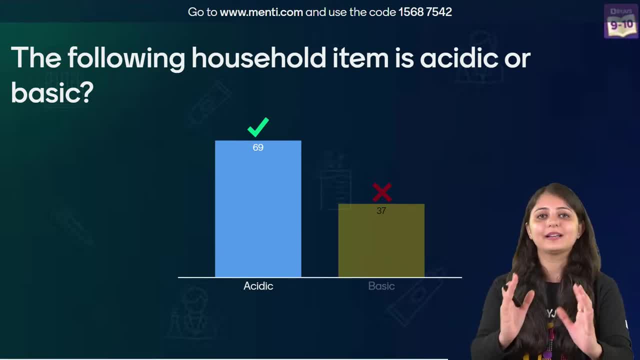 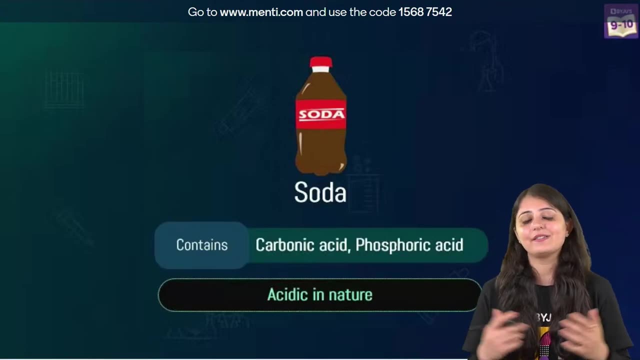 of answers here so i think this is a very good household item that has been placed over here this way you will actually understand what is present in soda so yes it is acidic in nature 69 of you got the answer right it contains carbonic acid phosphoric acid definitely it's 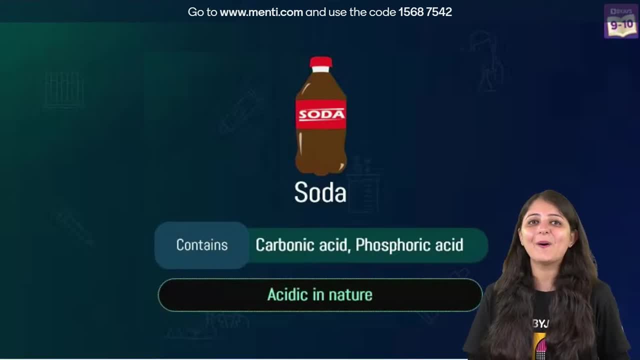 carbonic acid for phosphoric acid organic or mineral again correct awesome now you know the answer mineral correct okay is it are they weak or are they strong 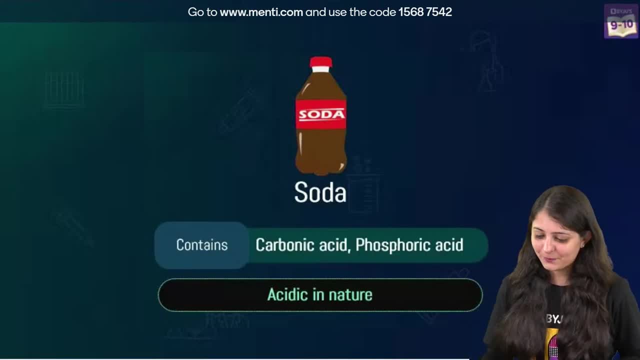 weak or strong quickly let me know 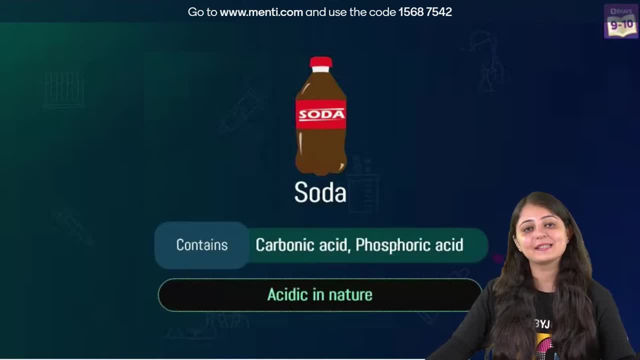 weak yes generally mineral acids are strong but carbonic acid phosphoric acid as we discussed yesterday there are exceptions chemistry is full of exceptions now so they are the exceptions and they are weak but yes super amazing performance and now you know your soda as well okay acidic 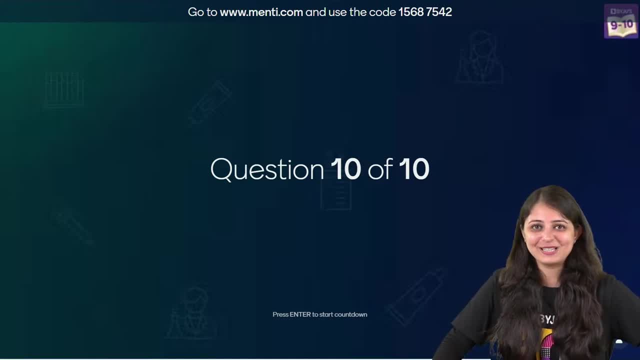 in nature up last question we are on to the last question guys last household item is going to come in front of you now 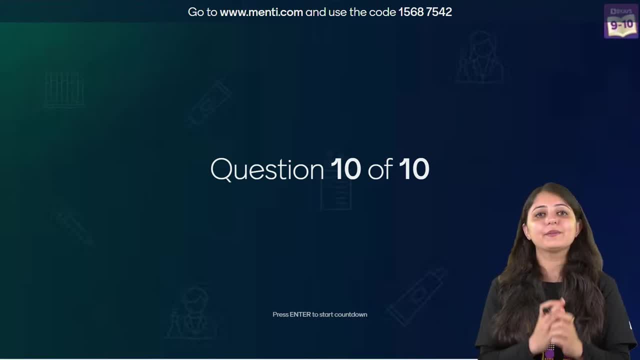 okay i want you to get this one right whatever your rank is i want you to in a way improve it okay that's why i was asking you about your ranks last household item on your screens now 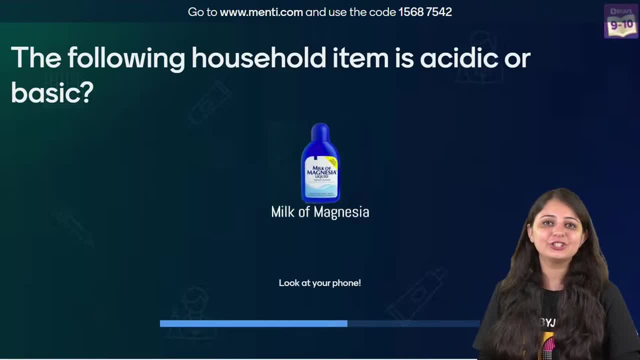 well it is milk of magnesia you might have heard about this you might not have heard about this let's see if you can answer this one correct milk of magnesia is it a milk of magnesia it's acidic in nature or is it basic in nature actually if you'll think where it is being used maybe you'll able to guess some of you are really happy yeah i'm telling you related with the use and then definitely you'll know the nature milli-year growth rates 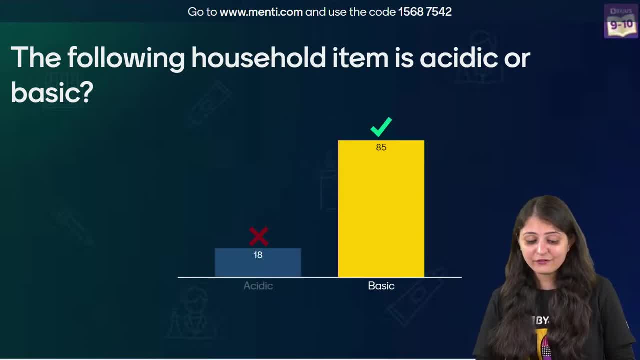 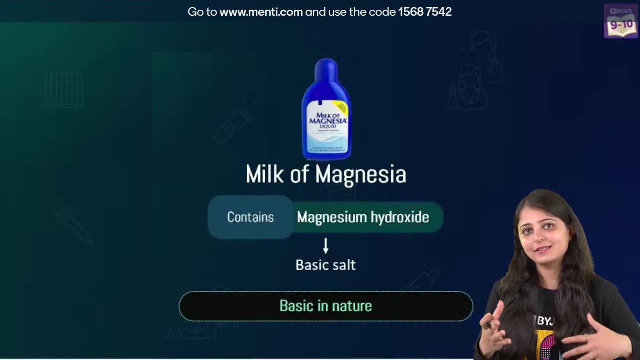 time's up and 85 of you have marked basic as the nature of magnesium hydroxide it's milk of magnesia which is absolutely right so milk of magnesia contains magnesium hydroxide so during acidity when there is excess acid to neutralize the effect we're using a basic substance a mild base that is milk of magnesia magnesium hydroxide and this is being used to 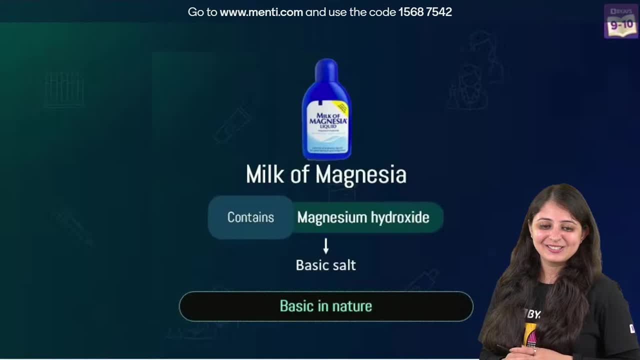 you know to cure the indigestion yes during acidity yes never it's mg oh hold twice 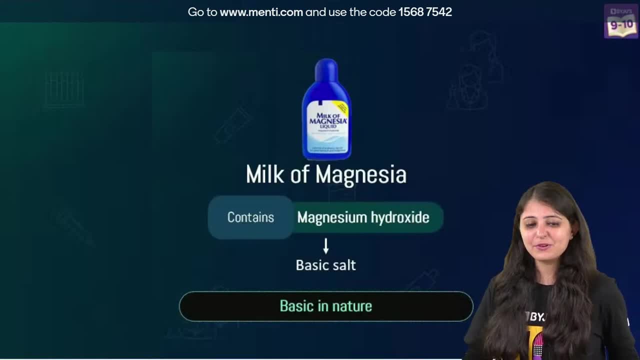 leaderboard priyanka is super excited to see the leaderboard 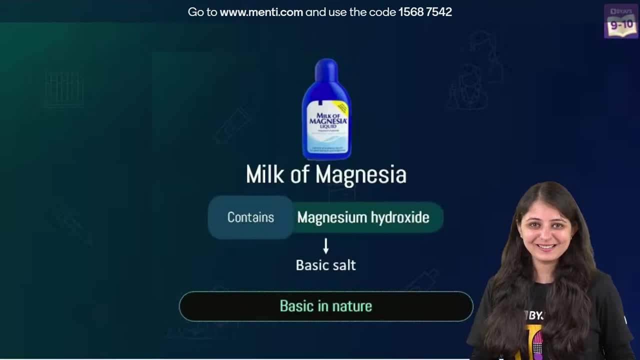 chalo load kare let's see how the leaderboard is looking now has the scoreboard presentation or the view has changed not changed hey anoop smart good one good observation but is it is it really visible is it really visible is it really visible kaha dikh raha hai hydroxide but okay nonetheless if you got the answer right that's amazing 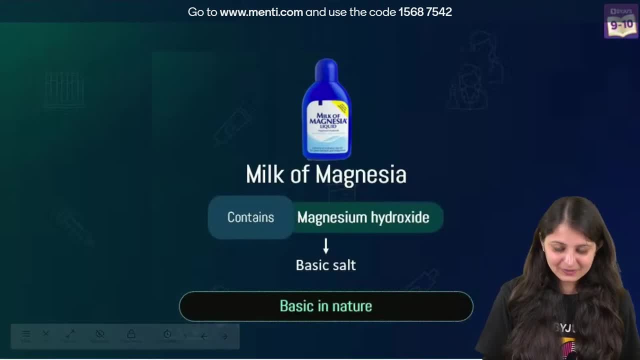 okay leaderboard now i want to see all smiley faces out there then i'm gonna load the leaderboard 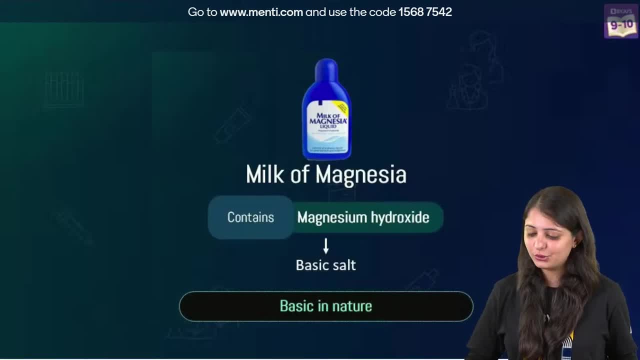 quickly give me loads and loads of smiley faces and then i'll show you the leaderboard 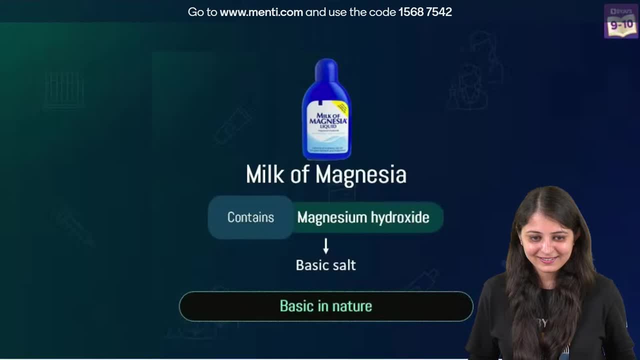 raj okay cool the chat box is looking amazing now let's load the leaderboard 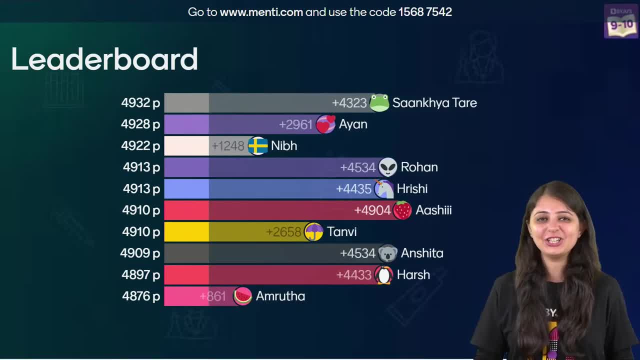 leaderboard and see has it changed not changed 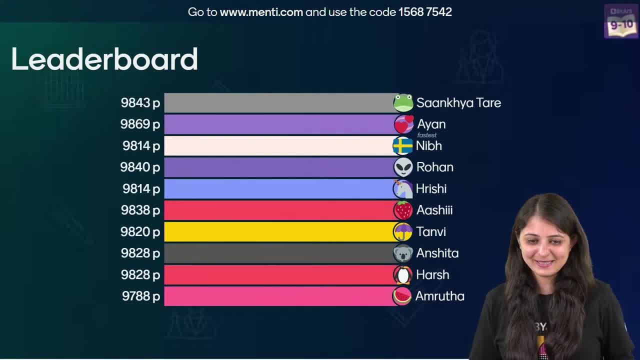 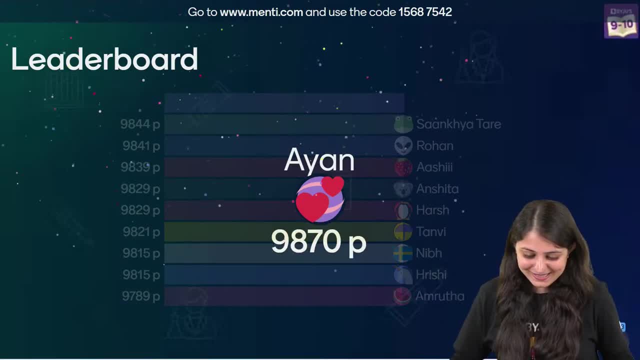 amazing amazing guys hey ayaan well done awesome sankhya rohan ashi anchita harshtanvi nibha rishi amruta well done guys well done yes ayaan is first dead of edit 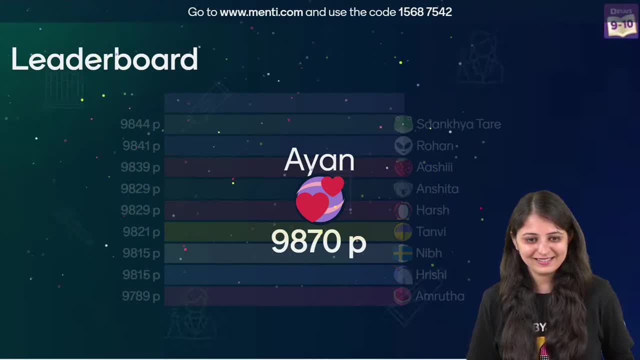 okay i want all of you to post your rank quickly great ya see some of you've improved your rank and that was the entire purpose for the second half of the mentee 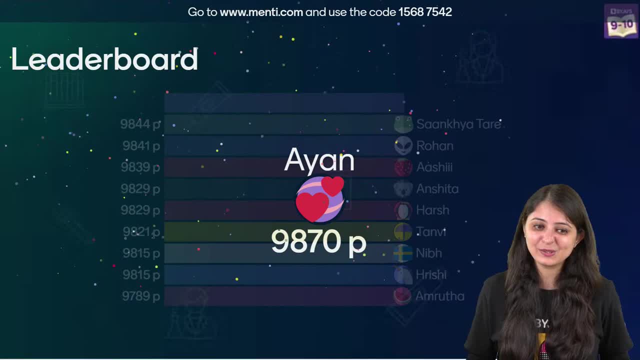 now you could just quickly improve your rank as well great yes omvir i can see that you are 13th from 90th to 73rd awesome yaar good job good to know that 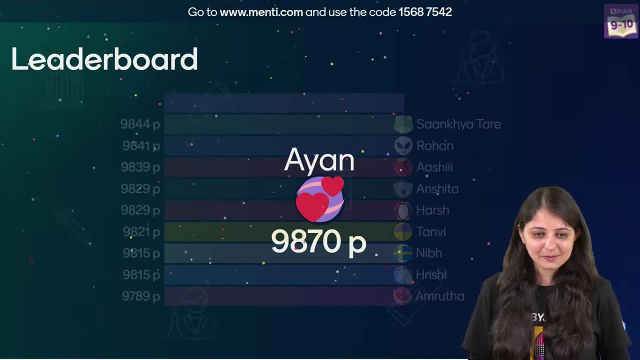 satyam is saying i am ayaan okay 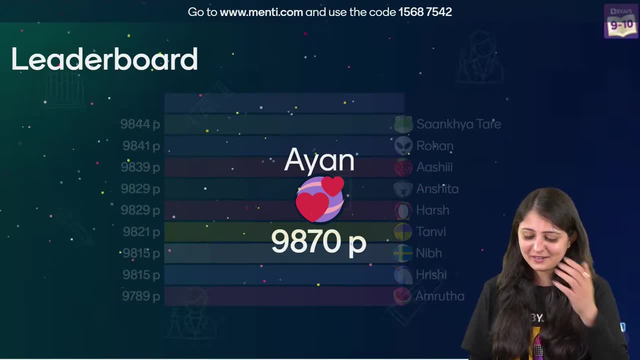 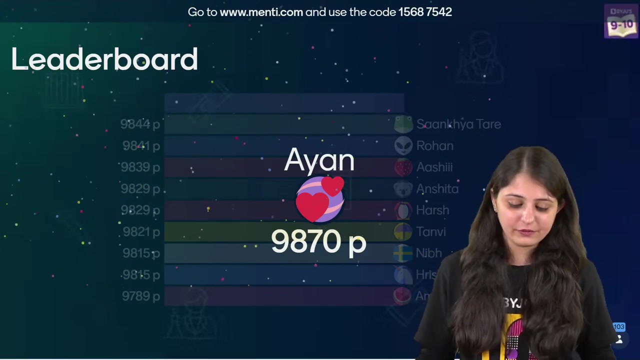 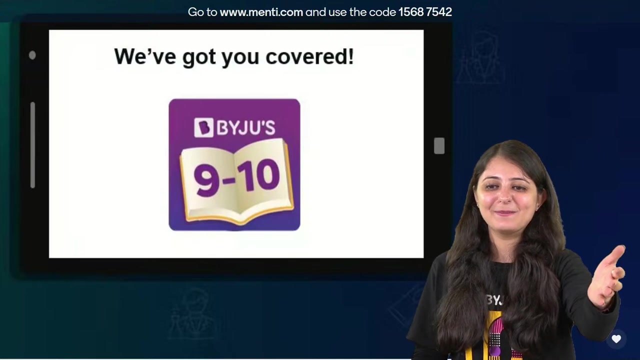 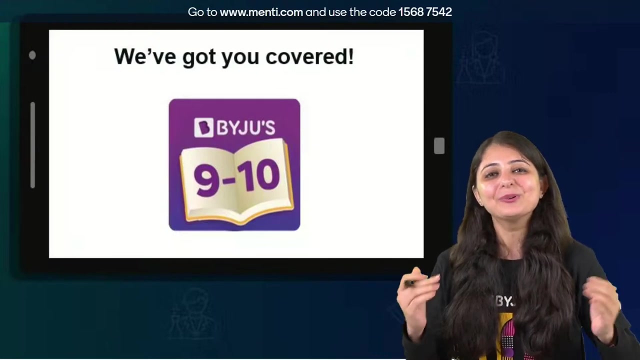 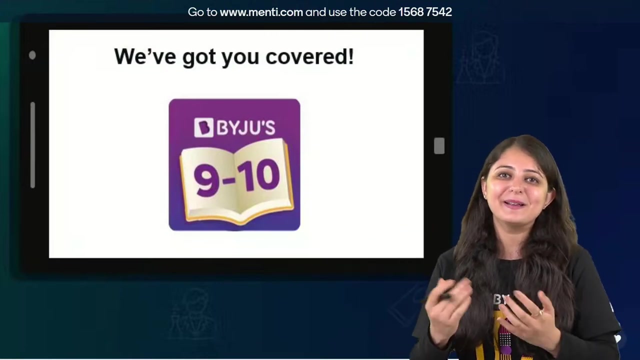 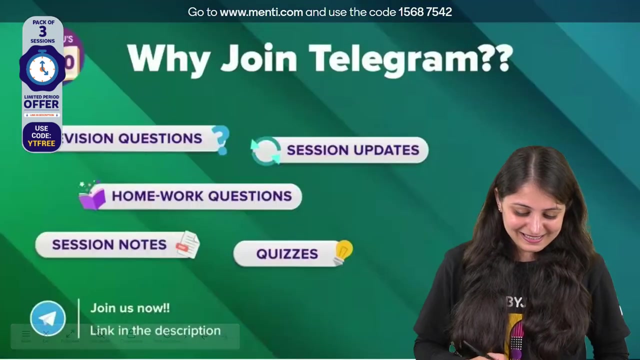 good great great great so if you've liked this session quickly first hit the like button so that we know that you love such mentee quizzes you love learning chemistry in this manner fatafat says video ko like kar do and give me loads of thumbs up over here great guys awesome really really wonderful performance by all of you so yes we've got you covered and i can see the thumbs up coming there thank you so much for being here i think it was a super amazing session i had a lot of fun with all of you i hope you also found the session super amazing super interesting and you've learned something out of it so now you know your household items a bit better great awesome so yes for the ones who've not joined take a look at the video and i'll see you in the next one bye bye bye bye bye 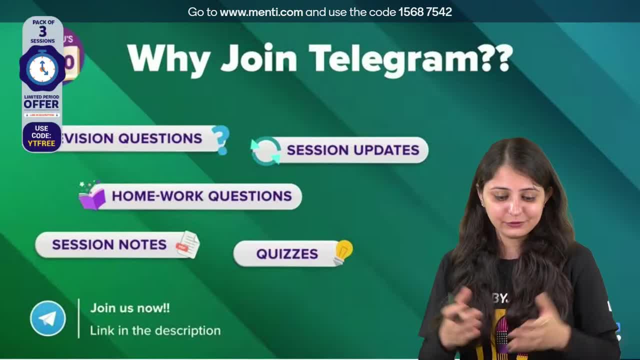 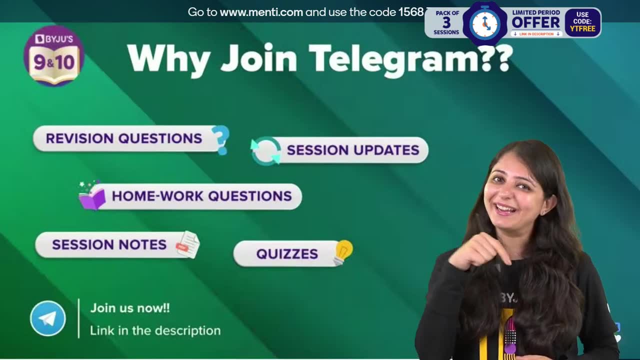 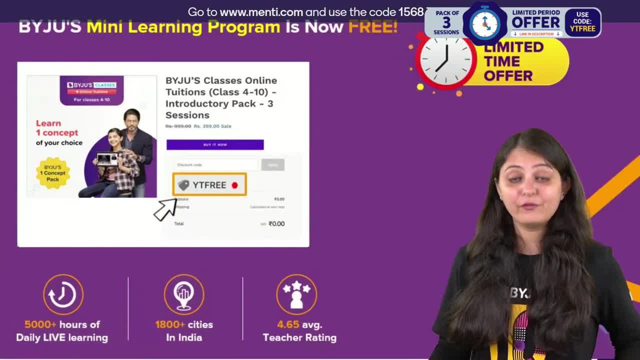